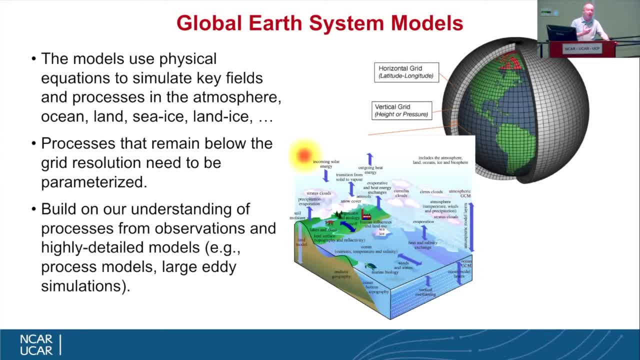 And they are trying to mimic the impacts of unresolved physics based on high resolution process models or based on observations and all of the parameterizations. Yeah, I don't think that I'm correct. I'm incorrect to say I'll just say: change it to most of the parametrizations, use resolved. 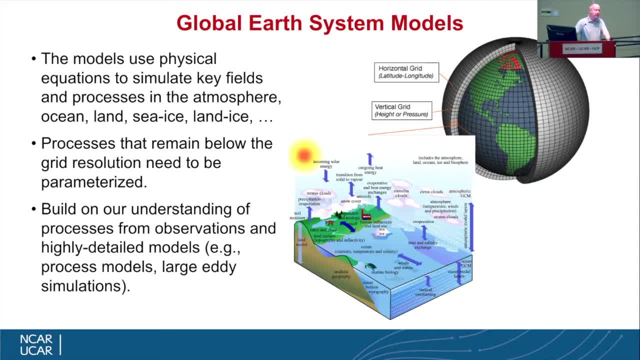 model variables to represent the impacts of unresolved physics or unresolved chemistry, And that's what we call parametrizations, and they require a lot of work. Some of them have been in development over 10 years, For example, vertical mixing schemes within the ocean model. 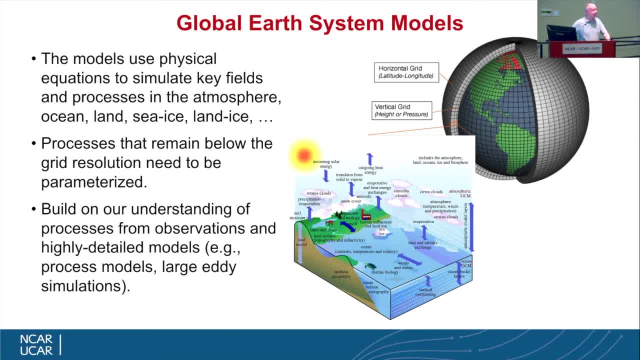 represent microphysics and you cannot clearly represent order, millimeter spatial scales. So all of those things need to be parametrized with the resolved model physics, And these representations are, as I said, building on process models. They are high-resolution models. 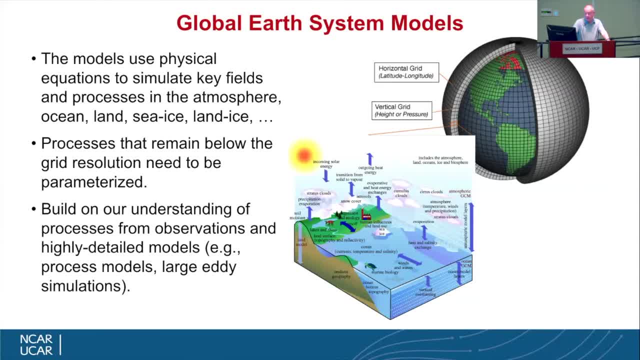 trying to represent those physics or observations or so-called largely simulations, And you can see on the lower right-hand side of the slide you can see that there are a lot of different models And on the lower panel here there are so many processes an Earth system model need to. 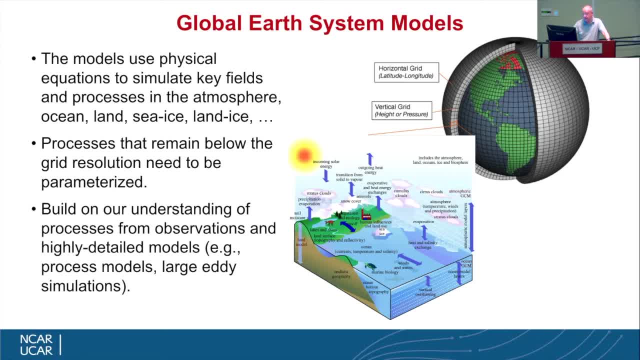 represent- And they are all I mean they are shown here- winds and waves. for example, We have a wave model. It represents actually explicitly impacts of waves. But if you look at the in the ocean interior, vertical overturning, that's usually vertical- mixing processes are not explicitly 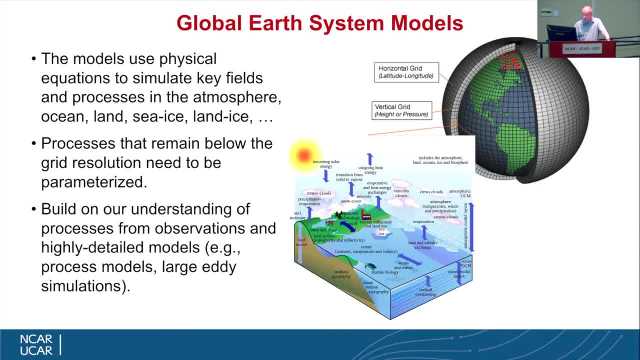 represented and need to be done, And so you know there are a lot of processes that are parametrized And, just to make sure that Peter is happy, we have land processes in the whole system as well. By the way, I forgot to mention that I'm an ocean modeler And, as Betty indicated, 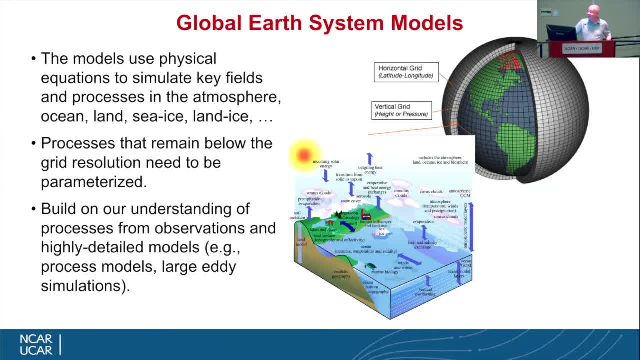 my background is quite different. also, My undergraduate is in mechanical engineering. My graduate degree, PhD, is in aerospace engineering. But the common thing between all of those is fluid mechanics and fluid dynamics. In engineering you don't have F as soon as you deal with the fluid dynamics. So you don't have F as soon as you deal with the. 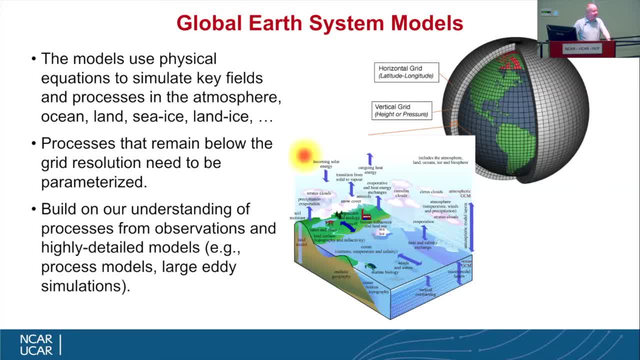 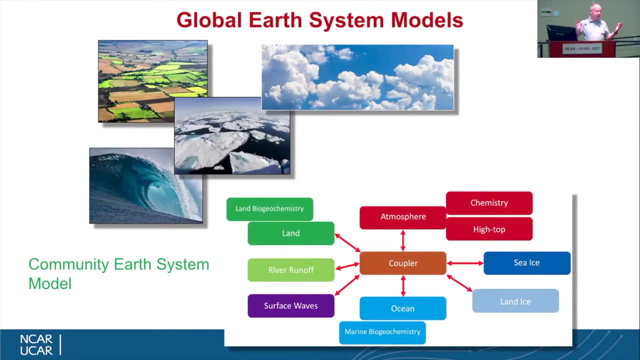 geofluidic, whatever the larger scale phenomena, then you have to include, of course, the Coriolis force. So that's one of the main differences. Okay, So global Earth system models bring all of the components, such as land, sea, ice, the atmosphere, ocean. We have the runoff also. 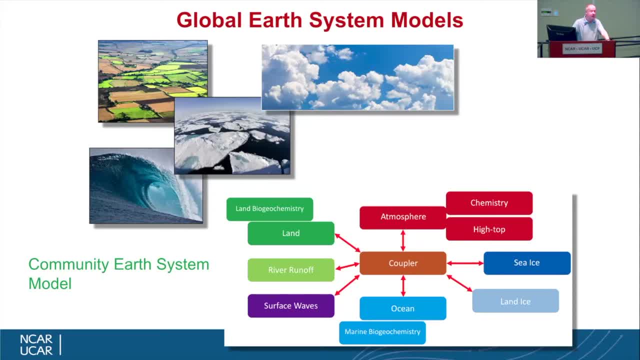 all of those components together And CSI is a global Earth system model And so you know community art system model and that he already gave sort of its history brings in all of those systems together and the schematic is shown here that we have at the center a coupler which is used 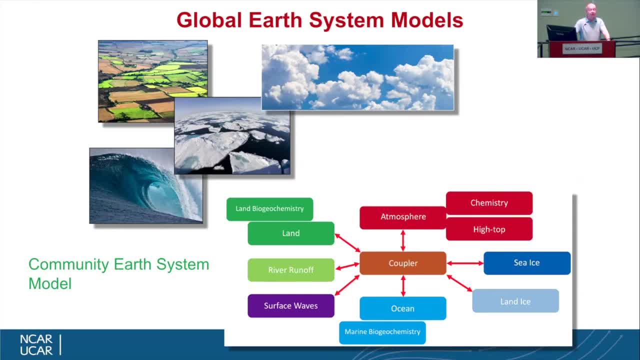 to exchange states and fluxes needed to drive each component model. we have the atmosphere model- we did this chemistry and a high top version that goes all the way to the troposphere, all the way- and we have the sea ice model. we have the land ice model representing glaciers, for example. we have 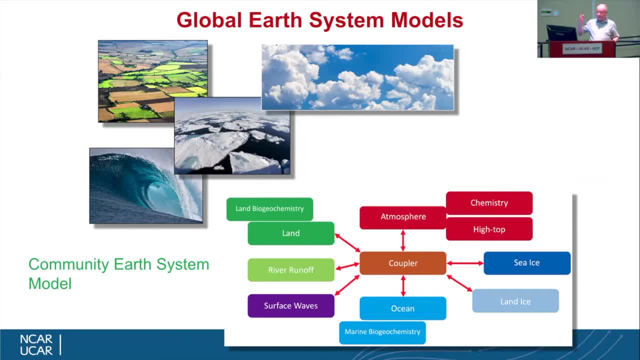 the ocean model and, since i'm an oceanographer, that's the most important component of the climate system. we have the marine biochemistry modeled within the ocean model. we have the land model and it's including its land biochemistry- river runoff and surface waves is included. 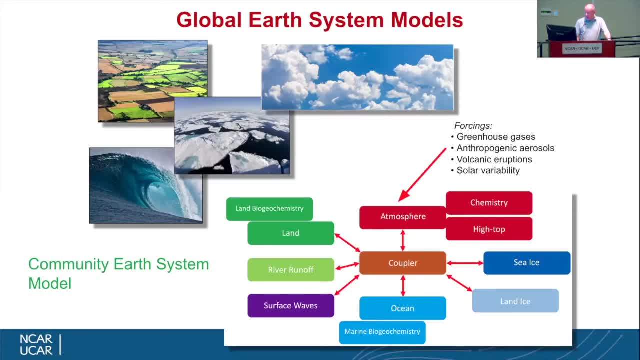 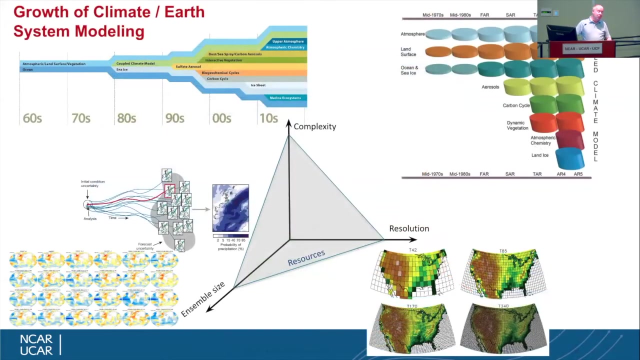 they're included in the model as well. so and then the? for example, in historical simulations, the four things are embedded in or provided to the atmospheric model. they can include greenhouse gases, anthropogenic aerosols, volcanic eruptions and solar variability. so one thing to keep in mind in global earth system modeling, or i think these are also true for 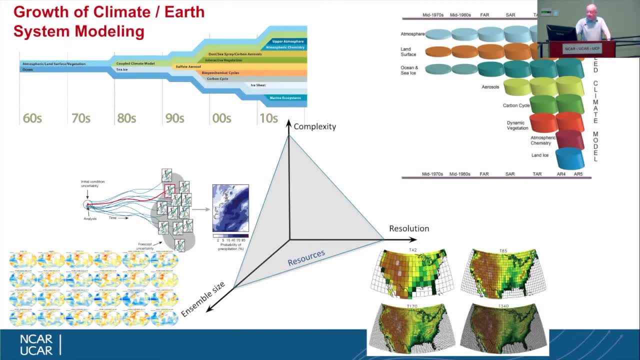 regional modeling system as well. there is generally a tension or competition between three things: model complexity- and it's shown in the center plot here- model model complexity, model resolution and ensemble size. and depending upon what your research question is and perhaps more importantly, how much resources you have, will determine what complexity what 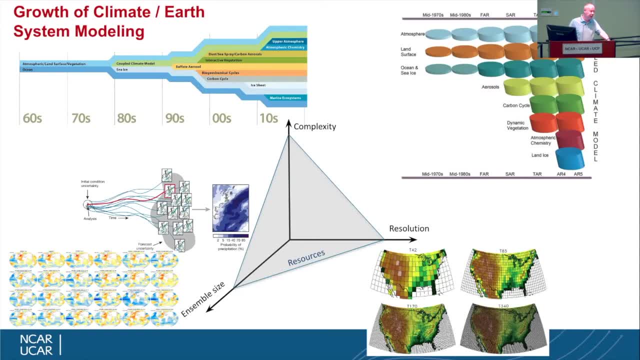 resolution and what ensemble size you would like to use in your research. so, uh, on the upper left plot here is showing the growing complexity of earth system models. when the sort of couple modeling started, there were only two components- atmosphere and the ocean- and for a while, for roughly two decades- nothing got added. but starting in late 1970s, additional 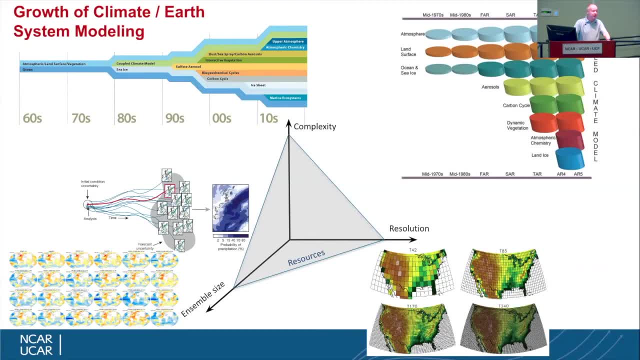 component models were included or started started to get included in the whole system and you can see that as we approach to the present that the thickness of that line grows considerably with additional components. another thing shown on the upper right here is that the as we include model components or missing components, previously missing components. 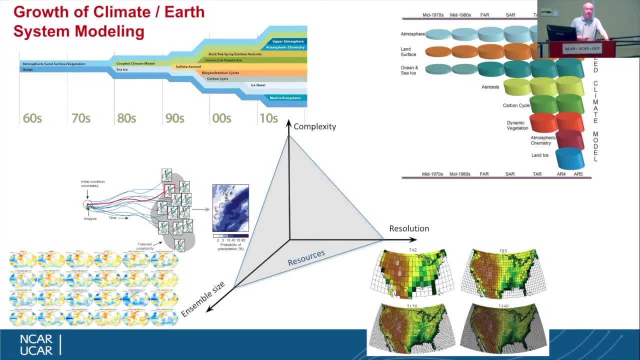 the models themselves are getting also complicated. we keep adding more features, we keep adding representation of missing physics continuously, and that's represented in the schematic by the thickness or the height of those cylindrical shapes. so they are also getting complicated. and then as we increase the computational power- uh, just human nature, i guess- we tend to go to higher. 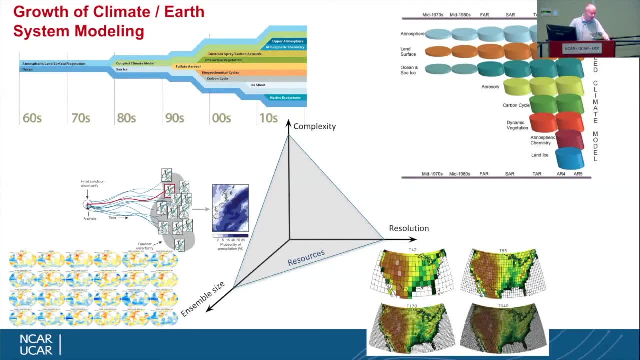 and higher resolutions. when i started working on climate models about 30 years ago- uh, i called it the real ocean, which was four degree by three degree ocean model with 20 vertical levels, and it was sort of the state of the art at that time and you can imagine that that's now not even 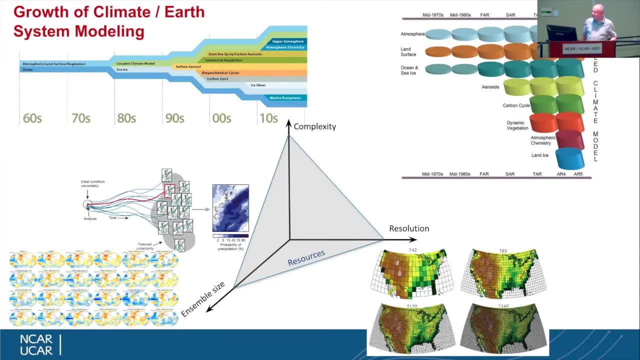 the standard for garbage, science or whatever, i don't know. the uh, so the the resolution. there's the desire to increase resolution as the computer, computer resources uh become more and more available. finally, in the past, uh again 20, 30 years ago, because of the lack of resources and all that. 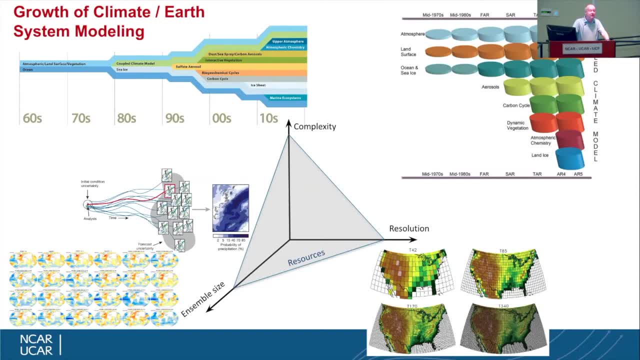 stuff. we were quite happy if we have one simulation of the historical period, because that's all we could afford and the ensembles or anything like that were just big dreams, and but now, with the additional resources and also with the realization that, uh, eat, i mean it's like the, if you just 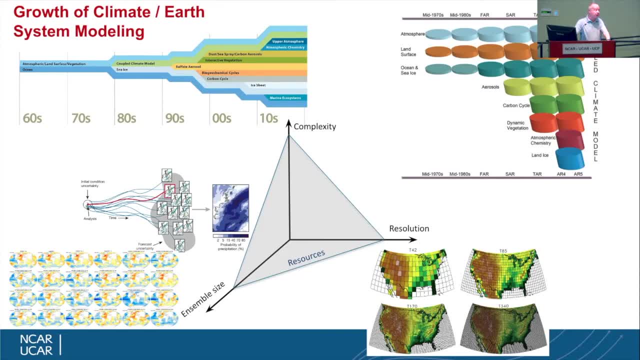 change, the uh change, make changes at the round off level. then you get substantial differences a few weeks later in the climate system. so people are now recognizing the importance of ensembles, and that's shown here. you start from an initial state seemingly very similar, uh, but then, as you integrate in time, it's just like the butterfly effect. right, it's just uh, the. 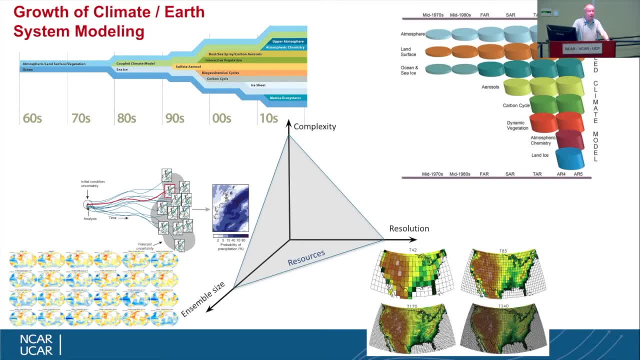 the paths of the system, uh, changes quite, quite a bit and then you get a huge ensemble, uh, spread in your fields. so, depending upon your science question, depending upon your research question, one of the first things that you are going to tackle in your research balance of these three, seemingly 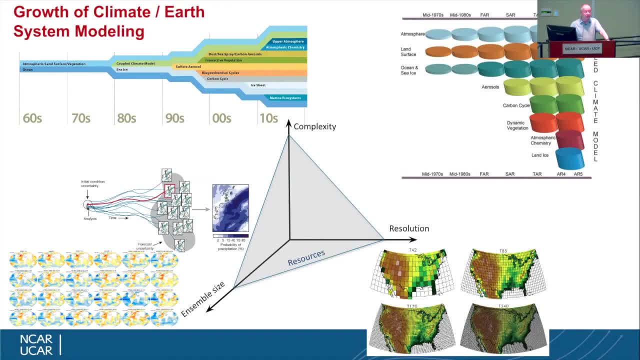 competitive things. you need to decide on the complexity of the model, whether your model setup is adequate to address your science. similarly, what resolution should you use and how many ensemble members do you need? and how many ensemble members you need strongly depends upon the question that you are asking. for some fields, maybe 10 members. 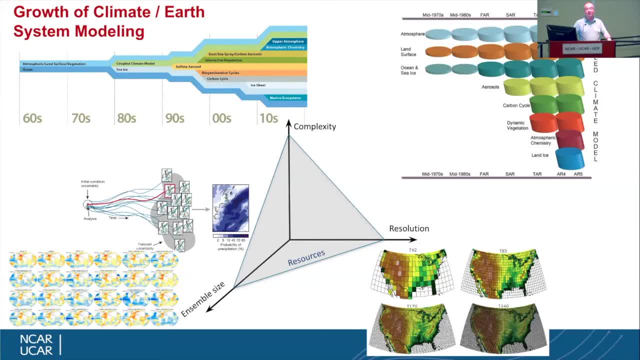 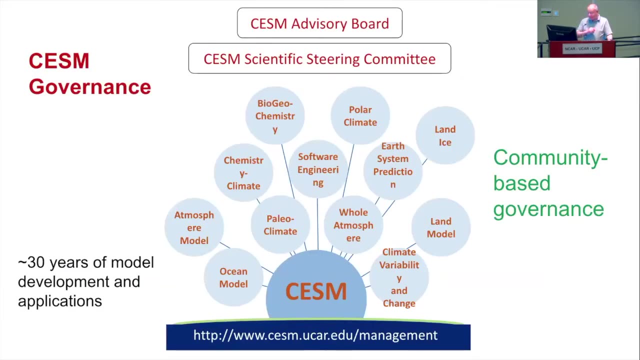 are enough, but for some other questions maybe 50 members will not be enough. So that's an important thing to decide And of course the big factor here is how much resource your time and the computer time you have. So, going back to CSM, I have no idea why this is showing up like that. 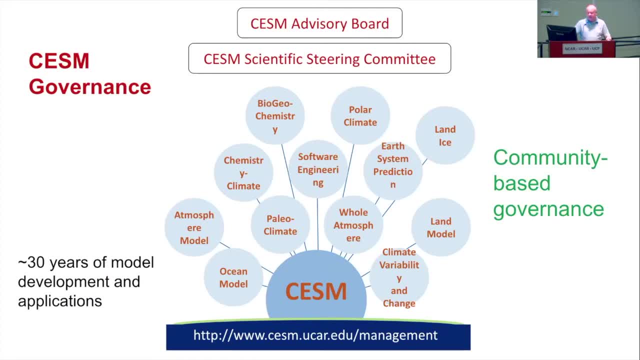 But anyway, Betty already indicated, CSM is we have been dealing. well, we've been actually involved with climate modeling over the last 30 years. It started in mid-1990s or early 1990s And I was lucky to be here at NCAR at that time when the whole thing started. 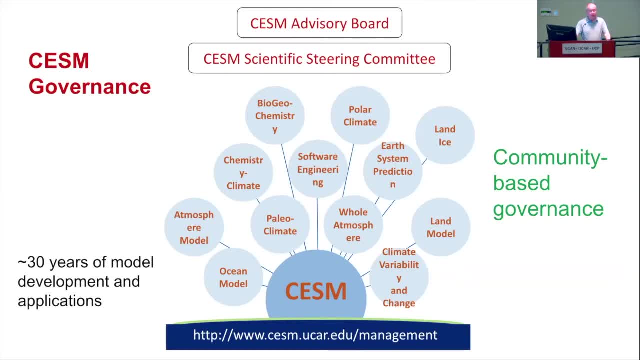 And today we have 12 working groups. Most of them are actual model development working groups, such as the atmospheric model working group and the ocean model working group or land model working group, But we have a few application working groups as well, such as Earth System Prediction Working Group. 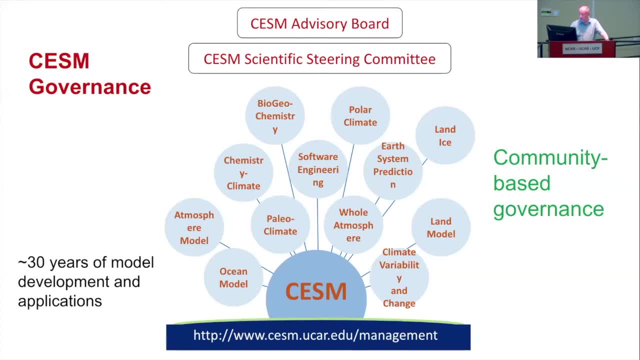 And Climate Variability and Change Working Group. The point of this slide is that CSM, as the C implies, is a community-based model And its governance reflects that All of the working groups have at least one non-NCAR co-chair. 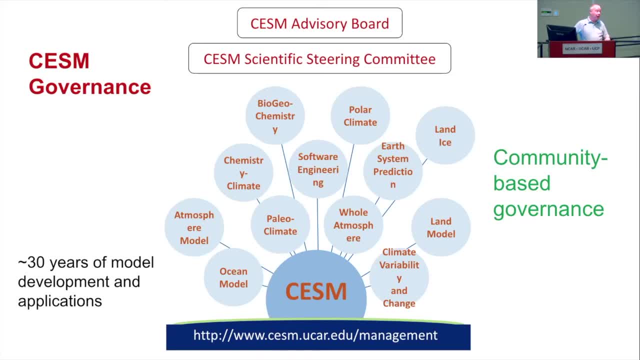 We have a CSM steering committee. of the 12 members, 10 of them are external. We all have a CSM steering committee. We have only internal members to NCAR: myself as the chair of the CSSC, and our lab director, Jean-Francois Lamarque. 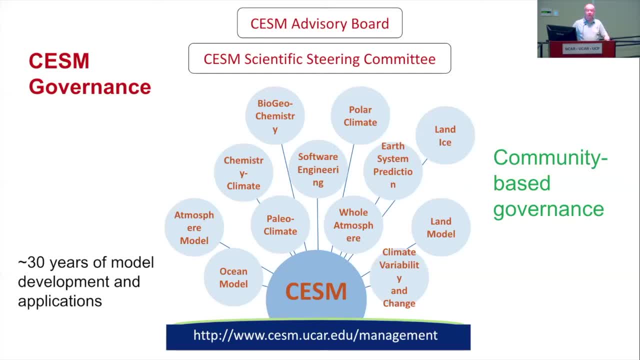 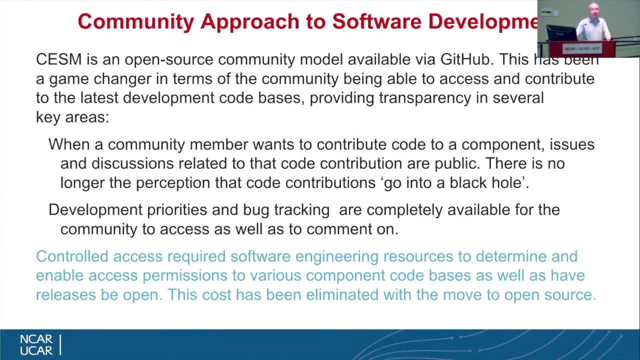 And we do have an advisory board which consists of completely external members to NCAR. So that's important to stress, I think, the community aspects. So we also have a community approach to software development. CSM: we have stopped releasing CSM. 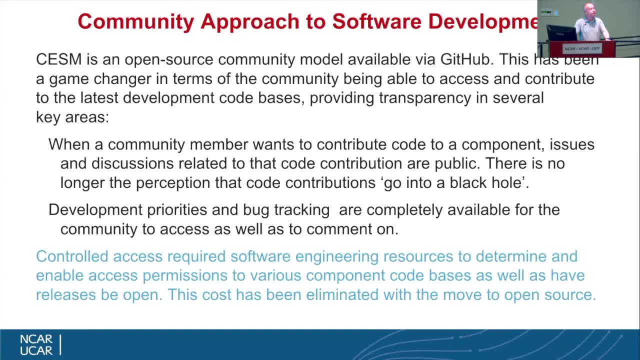 I think in summer of 2019, that was our last release- There is no such need anymore because all of the code is available as open source community model via GitHub. So if you want to see our latest model- not necessarily the greatest, but latest model version- you can access that via GitHub. 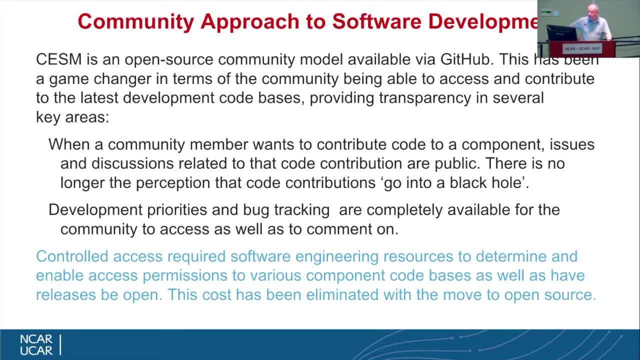 And this has been a game changer for us in terms of community being able to access and control. Thank you, So I'm going to move to the next slide, please. So this is a different approach. You can access the information in the community via GitHub. 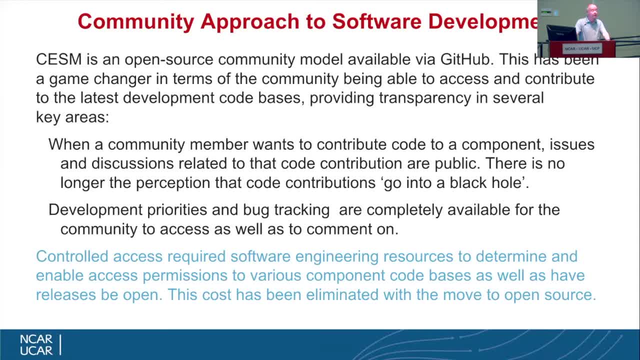 Right. we have a lot of support for community in the development in the development, So the community services can benefit from this approach. It's different from other methods that are out there, So we are using a lot of different methods. Yes, we are using different methods of place. 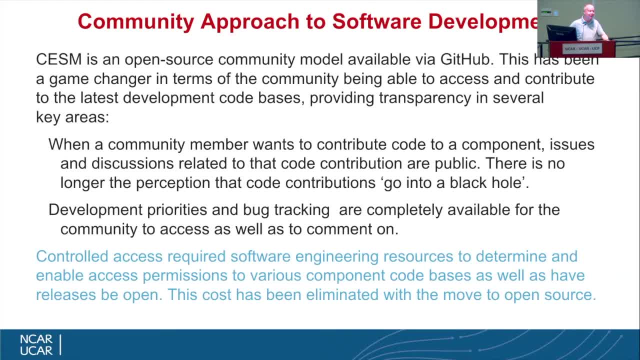 Right, three. Yeah, the first one is the performance, The second the next. Okay, somebody to control the access, make sure that people are aware of what the issues are, but with switch to GitHub, those are all gone. The downside of this thing is our sponsors, such as. 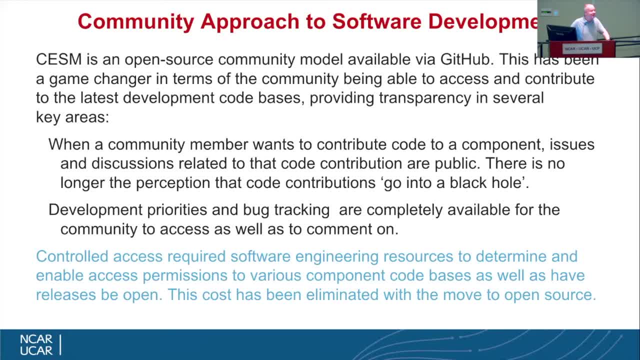 NSF would like to know how many people are actually using CESM and when the funding time comes. that's one of the first questions to get asked. but with open access policies, with the code base and with the data, and then with the privacy concerns, it's extremely difficult for us. 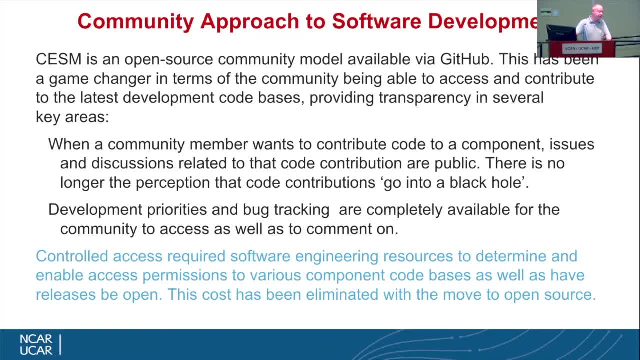 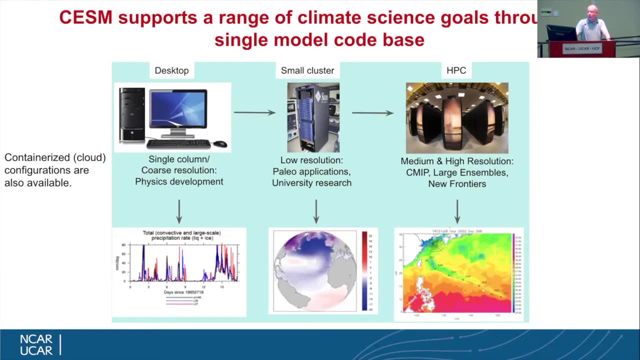 now to be able to pinpoint how many people actually are downloading CESM or downloading CESM data sets for their research purposes. So one of the success stories with CESM is that it supports a quite wide range of climate science goals through a single model code base. 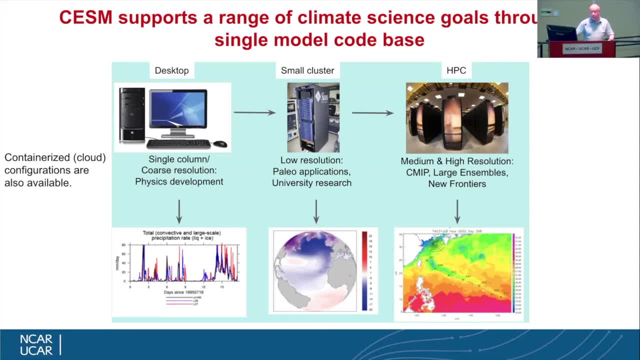 You'll likely see examples of the CESM code version on the cloud here. I believe in this tutorial, But CESM can be used on a desktop, for example as a single column model, and that can be used for parametrization development purposes. It can be used on small clusters. This can be quite 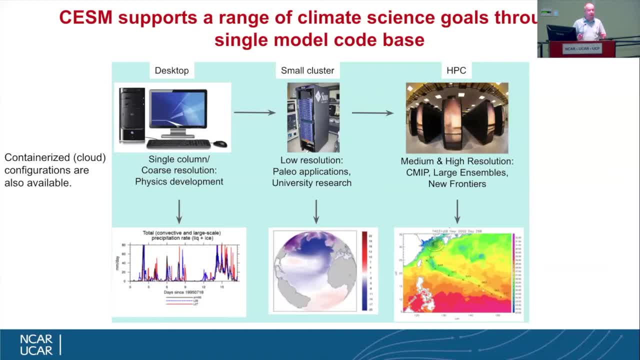 beneficial for university users to run the model on their sort of local system, and this can be run on course resolution and it can be run, for example, for paleo applications that require long simulations. And finally, CESM can be used on a desktop, for example as a single column model, and that can 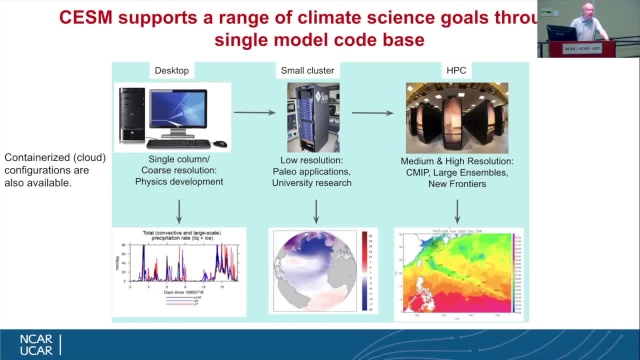 be run on course resolution and that can be run, for example, for paleo applications that require long simulations. And finally, on the other side, extreme side, it can be used on high-performance computers to perform what I call medium and high-resolution or ultra-high-resolution. 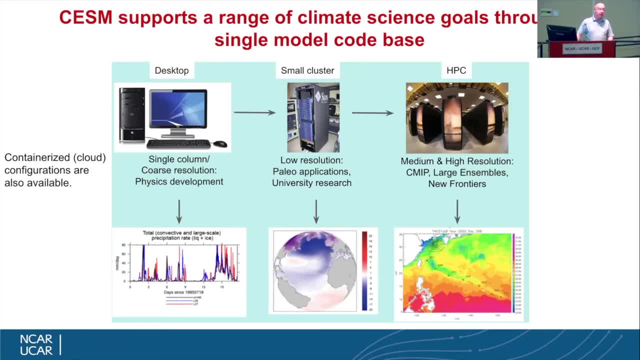 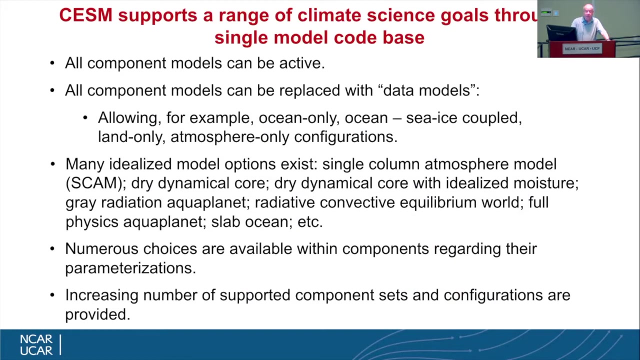 simulations. They can be used for a couple model intercomparison project purposes that contribute to IPCC that was mentioned earlier. It can be used for large ensembles or it can be used sort of frontier science questions, for example, See keeping up with the tune of sort of team of sporting, a range of science applications or 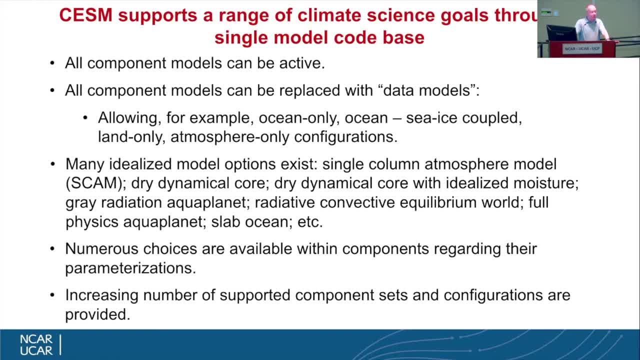 goals in CESM. all components, all component models can be run in active mode, So they're all fully active. All component models on the opposite end can be replaced with their data versions. So that means if you want to, for example, run the ocean model by itself, you can run it on a. 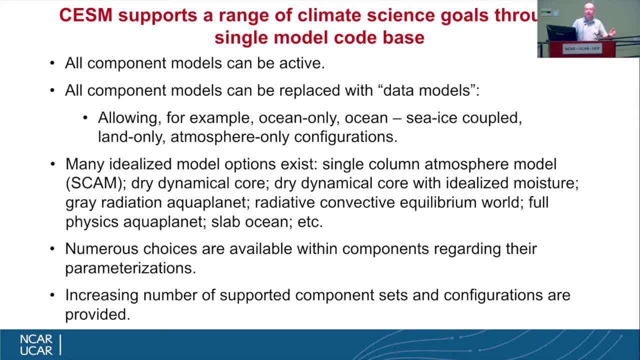 single-column atmospheric model. And then you can do so simply by providing atmospheric data sets needed to run the ocean model to determine the surface fluxes. We have many idealized model options within the system. Most of them are on the atmospheric side at this point, such as single-column. 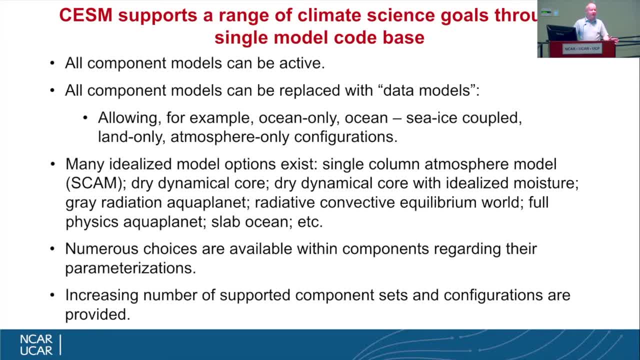 atmospheric model. I don't like the acronym, It's a SCAM model. I don't know why it's called SCAM, but anyway that's what it is. It can be used with different moisture properties. We have a slag ocean model, Although once, when you're an oceanographer, slab ocean is a four-letter word. 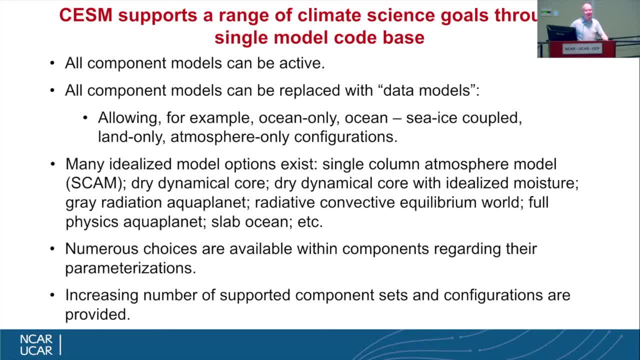 in the ocean modeling community, because we don't want an ocean model to be just like a slab model. We have numerous choices available within each component model in terms of their parameters and parameter settings, and every day, as I indicated on that complexity table, we keep adding more and more physics that were previously missing in the coupled system, so that increases. 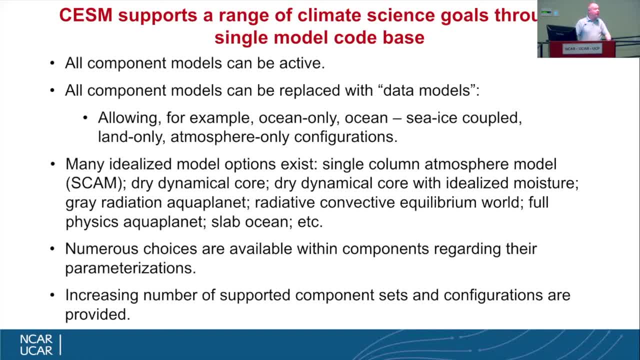 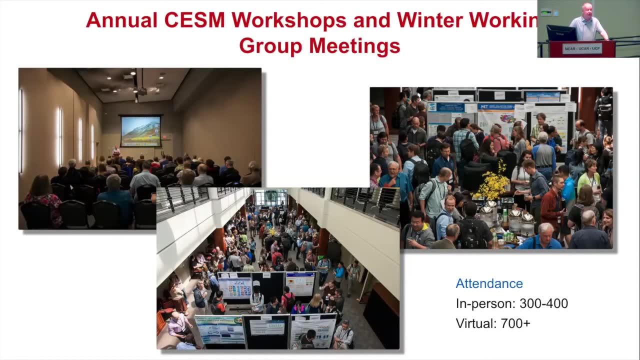 the complexity. But again, you can run it in simpler model configurations if that, if it is what is required for your research. So, in terms of community engagement, CSM writing is one of the- I think it's the only model- the climate modeling community- it is truly a community model and we have annual workshops. 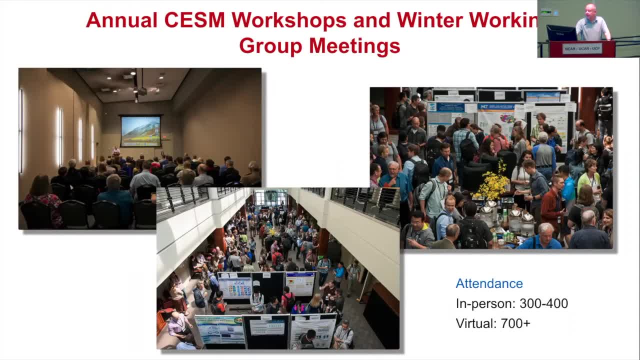 they happen in June usually, and then we have each working group also their winter working group meetings In person. when we have the annual workshop in person, we had three to four hundred people attend that and this room was one of the venues and we had probably three to four hundred people sitting in this room without the desks When we switched to. 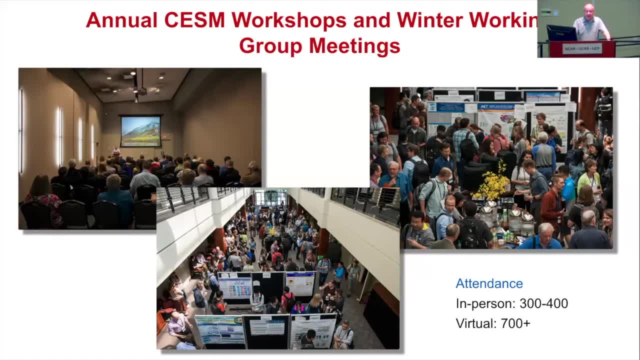 the virtual environment. during the past three years our attendance went up to seven to eight hundred people, but it is difficult to judge how engaged that group is- usually people, as you know- with the virtual environment. you do 10 things at the same time and your attention is really not much for one. 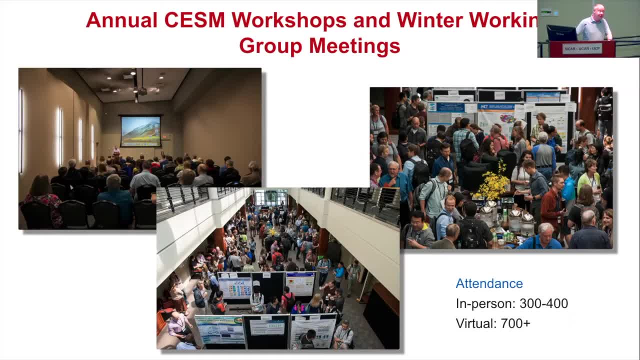 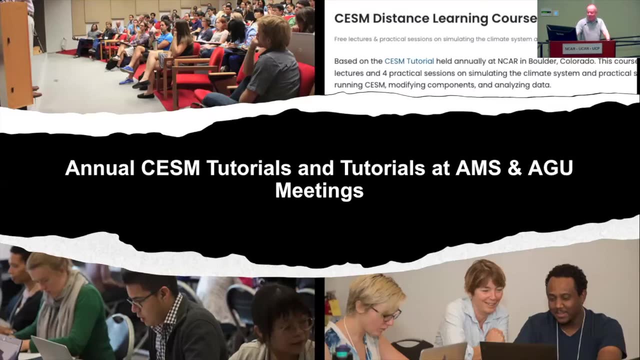 of these things, so the productivity and creative creativity goes down, go down quite significantly. so that's why I think it's important to have in-person meetings like this. Okay, and then another point of being a community model: we have tutorials and this is the CSM annual. 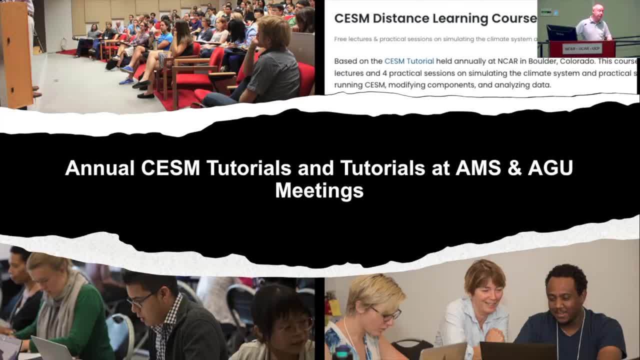 tutorial. We do also have shorter versions of this tutorial meetings. they run either half a day or one day and they are sort of compressed versions of these. so if your friends or if you are still interested in learning more about the CSM, you may want to. 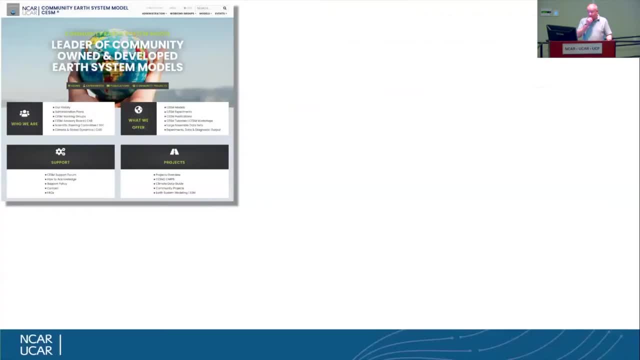 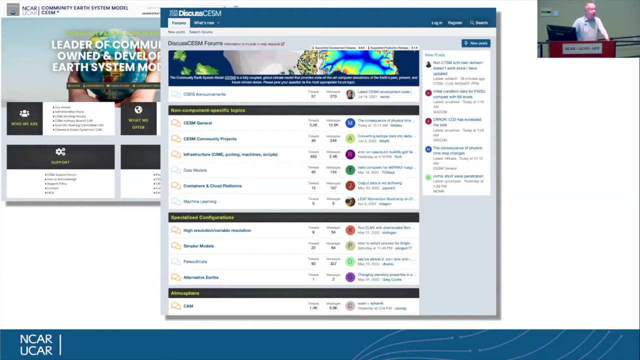 take a look at those tutorials and you are probably already aware of our web presence. Many of the tutorial materials are already on the web and, as a community model, we need to be also cognizant of community needs. community has a lot of questions and we have forums. they are answered and this is 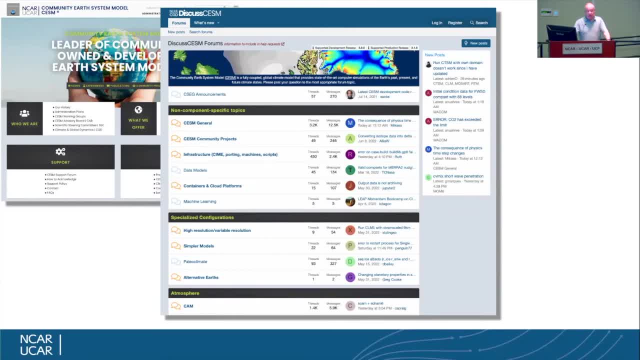 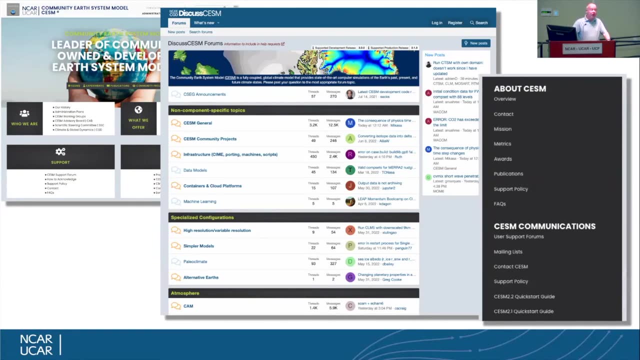 just an example of this. this is showing what kind of questions can be asked or are being asked and they are being answered, and the community members can answer these questions as well. and then we have also lots of documentation in terms of model use, how to name your experiments, how to name your data. 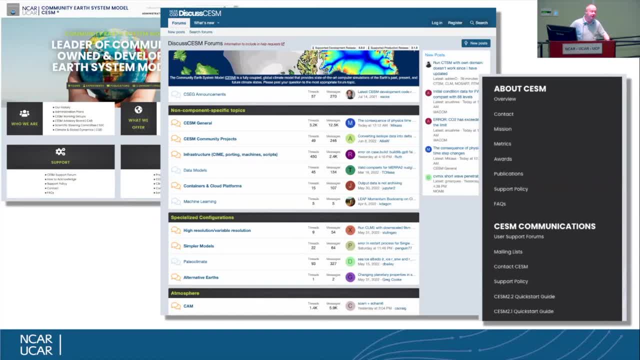 and I just also recently updated the CSM data policy and you may want to also take a look at. take a look at what it says in terms of what we can store and what needs to be stored, perhaps with respect to model output. Okay, so this was sort of a brief introduction. 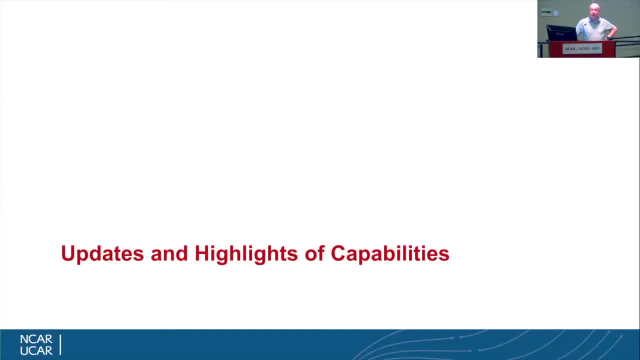 to our capabilities and our community sort of engagement efforts. do you have any questions so far? okay, so if not, I will try to now, in the second half of the presentation, try to show you some of our recent efforts. I'll try to show you some highlights and also try to answer some of the 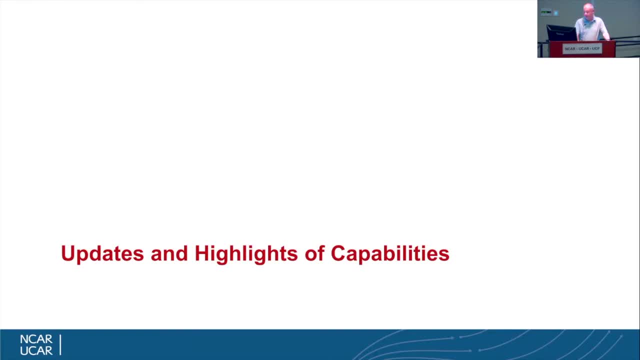 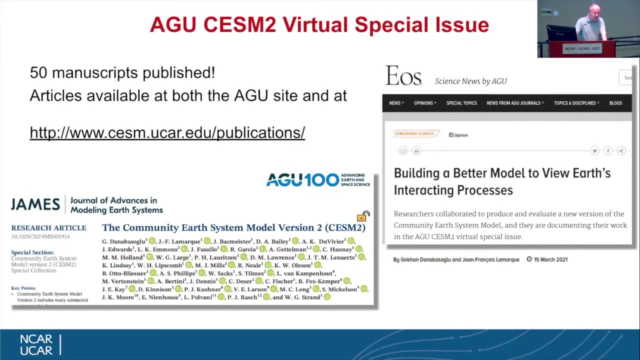 questions with respect to equilibrium climate sensitivity, which is an important topic. I think so. as we mentioned before, one of the activities or one of the efforts that we do is to participate in a coupled model intercomparison project and those the results from that project or those simulations. are you familiar with the coupled model into comparison project? that's the latest. 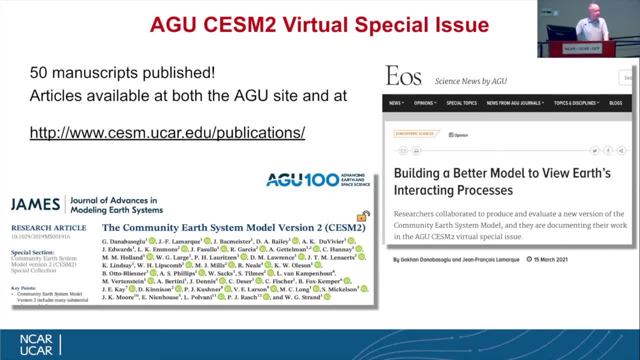 effort, the CMIP6, and it is asking for coordinated simulations from interested modeling centers. there is a deck set of experiments. they are mandatory usually and there are multiple order 20 to 30 or even 40 MIPS modeled into comparison projects sort of. they are satellite MIPS around the deck simulations. so that was one of our major activities over the 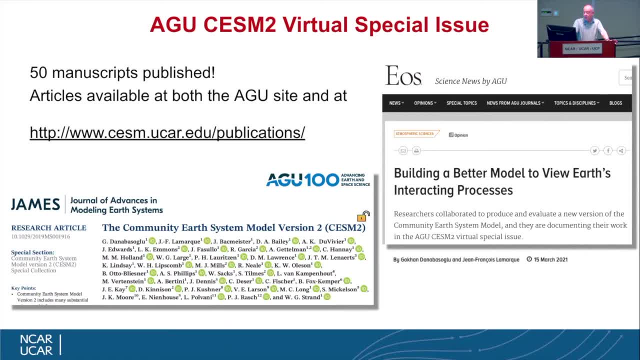 last five years or so and we have arranged for an EGU-CSM2 virtual special issue and if you're interested in learning more about these experiments, please do so. simulations and their analysis: you can go to that publications website or you can just go to also. 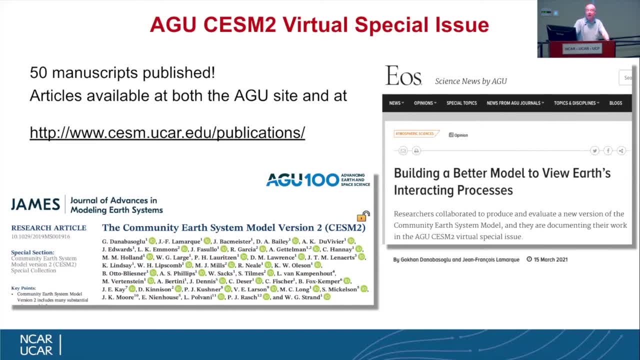 EGU website to access all 50 manuscripts. they are published and they are all free access, so you should be able to access them without any issues. I just included the primary manuscript here that was published in 2020 and then last year, early last year, Jean-Francois and I wrote an article or: 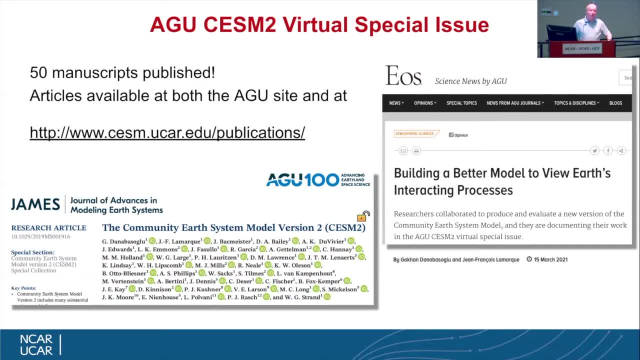 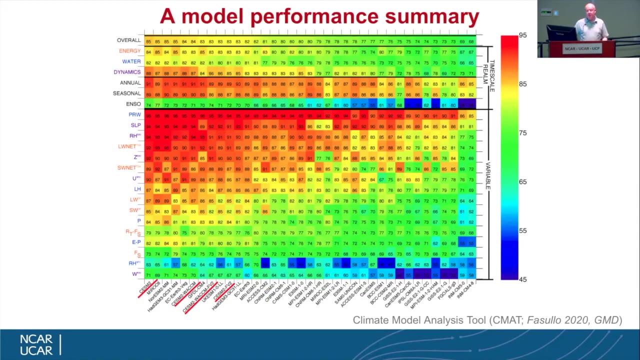 opinion piece in EOS to introduce the special issue as well, and I think that's, if you're interested, and that's a short article that you can just quickly learn about challenges that that we encountered during this development process. So one of the successes of CESM is that it is collaborations with the community, not just within. 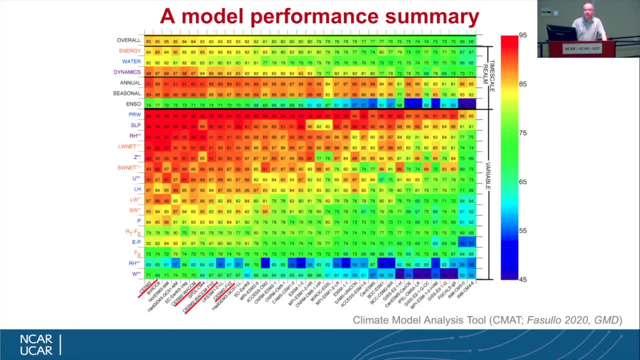 the US碰 the United States, but also external community, And we get quite a few requests for collaborations And I believe that the reason for such requests is the model fidelity of CESM, its simulations, And I'm showing an example here from John Fosullo. 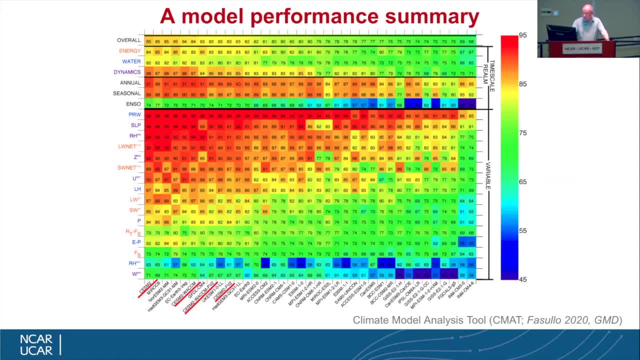 it's published in GMD. He has developed a toolkit called Climate Model Analysis and this is showing a summary of model performances across roughly 35 or 36 models that participated in CEMEP6, considering energy, water cycle and model dynamics, And those are color coded. 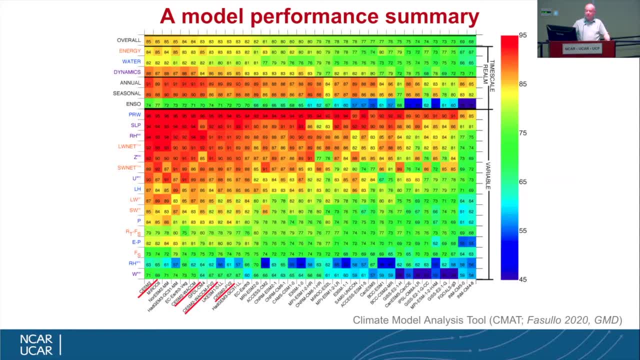 The fields related to energy are in, for example, orange, fields related to water cycle are in blue and the dynamics related fields are in purple. And then, compared to observations and compared to reanalysis products, a score is given and it's considering the mean annual cycle. 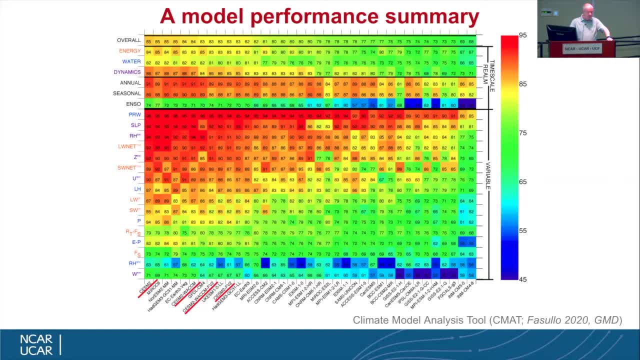 and some short-term variability. So, and then there's an overall cycle, overall score at top as well In this plot: if you are on the red side, it's good, If you're on the blue side, it is bad. 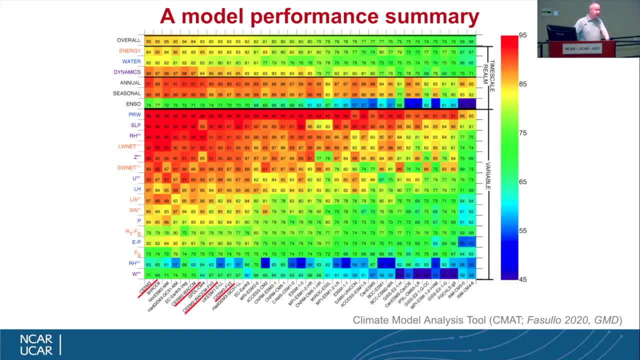 So you can see that I underlined we contributed with 10 model- sorry, four model configurations to CEMEP6 and I underlined the ones that are associated with this CESM. So I was quite happy to see that if we are in the top 10. 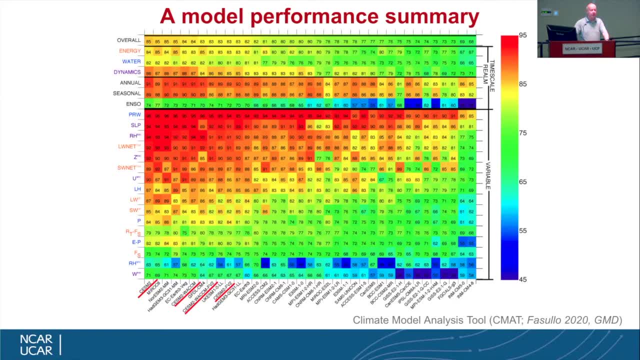 with all of our four configurations. So I mean some people don't like models into comparison projects, sort of a some kind of context: my model is better than yours, but it has it. it has some benefits. it can expose model errors and all that stuff, but in this case i would like to stress that 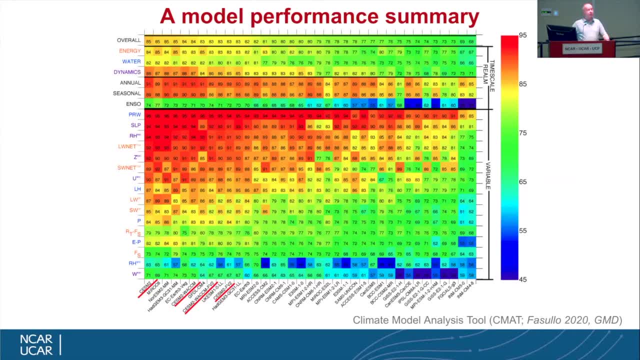 when we get collaboration requests from external part, external folks and all that stuff. this is one plot they tend to look at to recognize the fidelity of cesm and it is solutions. so that's, i think, an important aspect to stress how many of you are familiar with equilibrium climate. 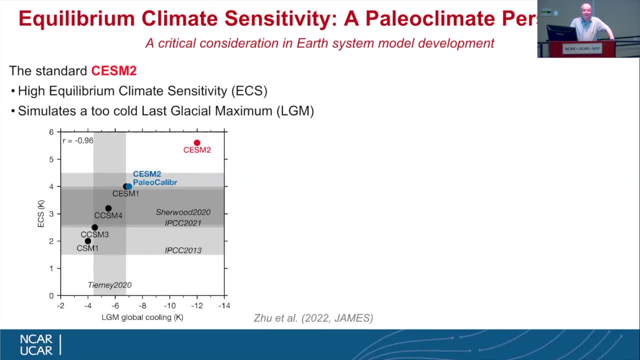 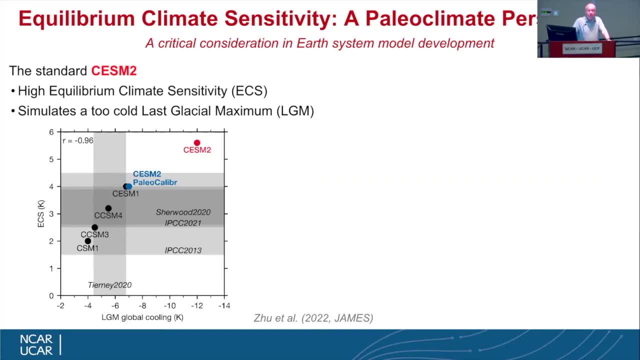 is to a doubling of co2 concentration, instantaneous doubling of co2 concentration and how high the uh, uh surface temperatures go up. so it's a measure of sensitivity of the surface temperature to increase in co2 doubling. but when i say hypothetical equilibrium is in the in the phrase equilibrium, climate sensitivity, clearly, in order to get to. 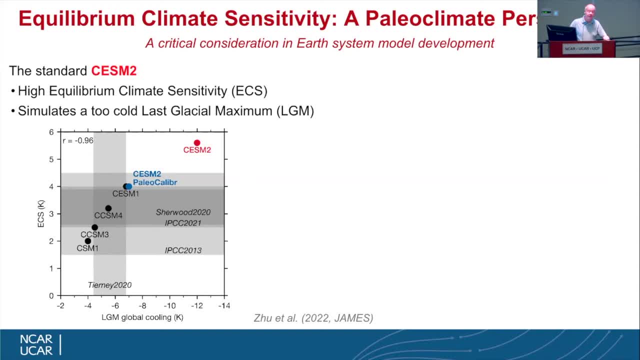 equilibrium, you need thousands of years because of the diffusive time scales within the ocean model. in this case, it represents an estimate of equilibrium climate sensitivity and, if you are familiar with gregory et al methods, it's essentially an extrapolation of a regression line and it's usually referred to as effective climate sensitivity. but in any case, 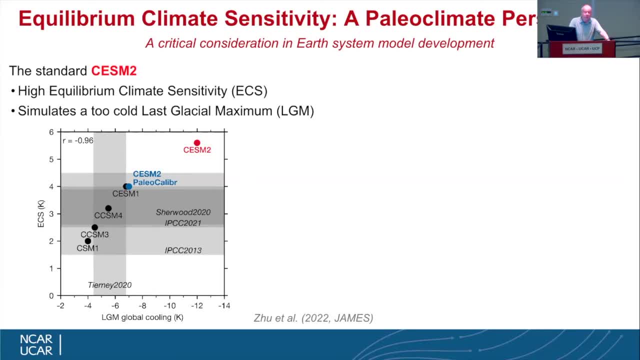 cesm is one of the, was one of the models, or is one of the models, with a large equilibrium climate sensitivity about five degrees celsius. we don't know what it is, but the accepted range is usually around four to, i don't know, three and a half to four and a half degrees celsius or so, and it is I. 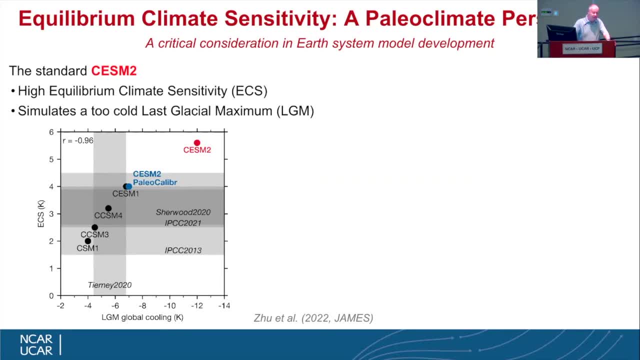 mean it is. it is some uh. these estimates are based on some paleo climate approximations or uh records as well, but in most cases it is. people think that it shouldn't be less than and a half perhaps and it's. if it is more than four and a half maybe it's not the right value. 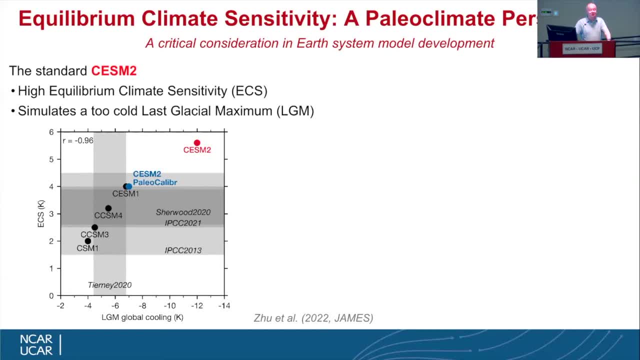 so it is sort of an expected range. i would say it's not that's what people want to see the equilibrium climate number to be. so our climate working group spent quite a bit of time trying to figure out how the present model setup would behave under last glacial maximum simulations. 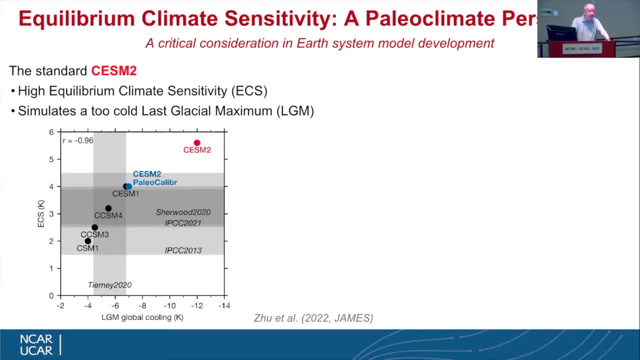 what is shown here is a scatter plot of the last glacial maximum global cooling for surface temperature, plotted against equilibrium climate sensitivity you can, and then the shaded regions are estimates, the vertical one and estimate is estimate from the paleo records for the surface cooling, and the horizontal lines are the ranges for equilibrium. 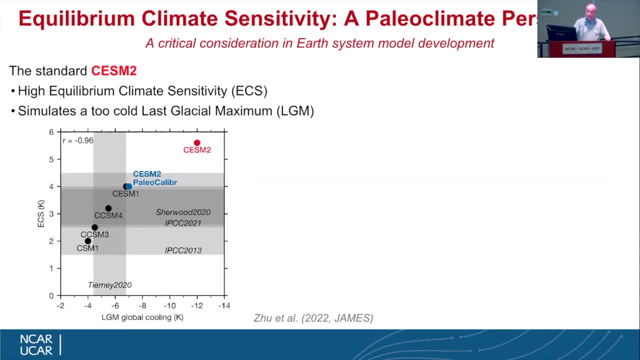 climate sensitivity from ipcc reports. the previous model values were along the you can see here is a scatter plot of the last glacial maximum global cooling for surface temperature. the csm model versions are shown by the black dots here, so they were within these estimated ranges. 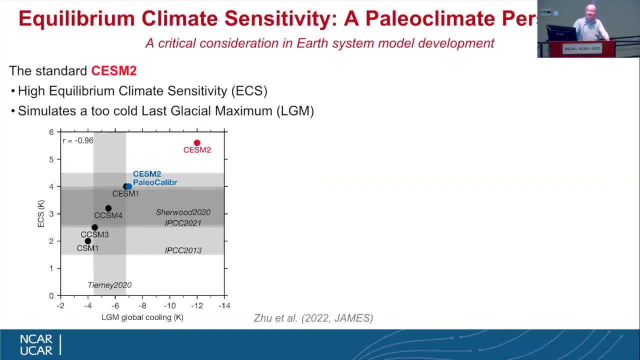 but you can see the csm2, which is the red dot there. it is outside these the. the point here is that maybe equilibrium climate sensitivity is not that important, but when you run a last glacial maximum and if your surface temperatures are minus 12 degrees, as opposed to be less between minus five, 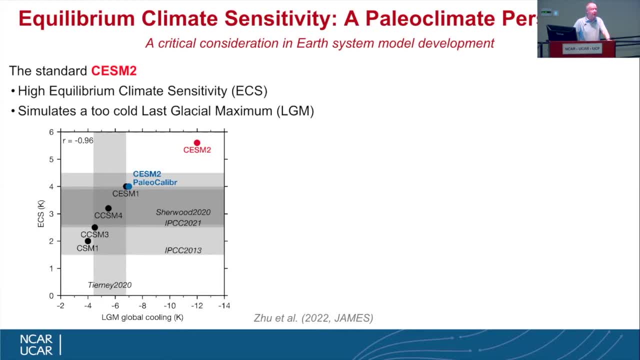 and minus seven degrees and you run a last glacial maximum and if your surface temperatures are minus seven degrees celsius then that's a problem. so they went back and checked, spent roughly two years and looked at cloud feedbacks- aerosol cloud feedbacks- and they found that a particular 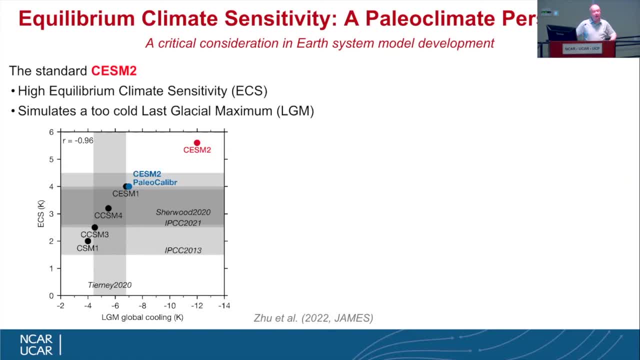 parameter setting in the microphysics scheme in the atmospheric model related to mixed phase clouds. it was limiting the number of ice particles in that scheme and once they took that limit away- and it was my understanding is it was there inadvertently- once they took that limit away they obtained the blue dotted line. so you can see that both the last 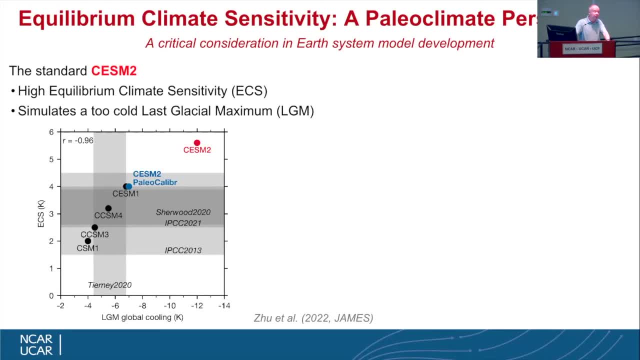 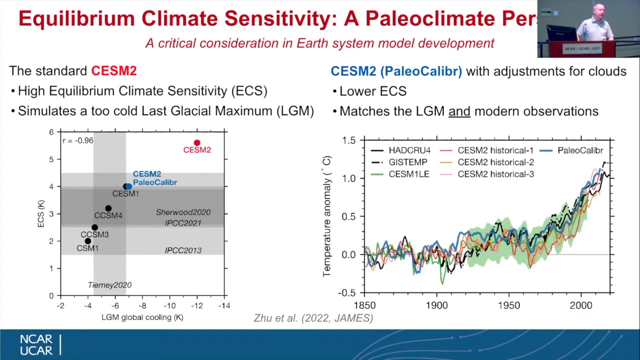 glacial maximum, surface cooling and equilibrium, climate sensitivity went down quite significantly, so now this version of the model is within accepted ranges. of course, last glacial maximum is okay, but then you have to also look at how it's behaving in present day or historical simulations. so the new simulate- what is shown here- is the. 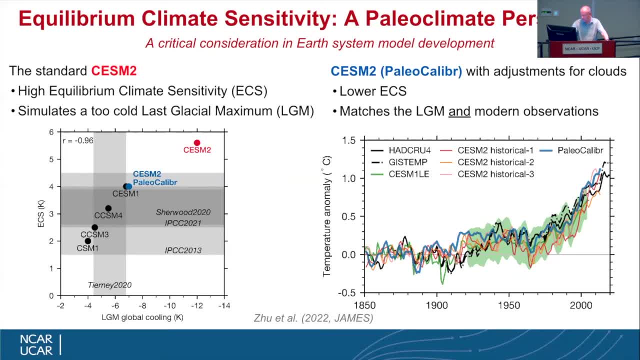 temperature anomaly with respect to the. i think this is for the 1850 to 1900 period of the surface time series. surface temperature time series anomaly time series. the observational time series are shown by the black lines. other lines are showing estimates, other lines are showing the previous model versions, including csm-1 large ensemble spread, and then you can. 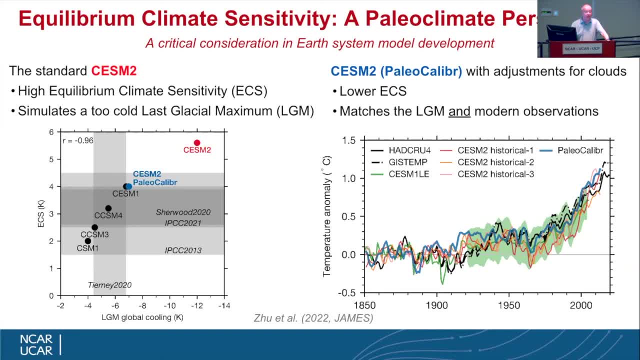 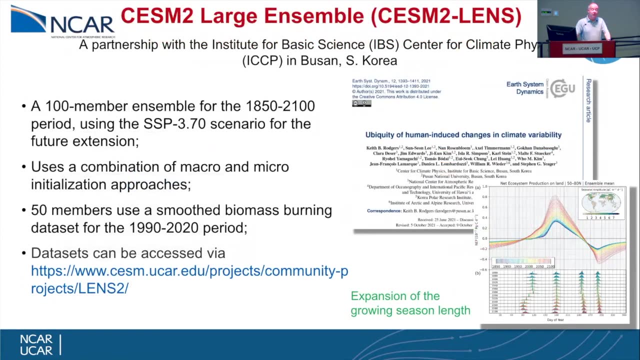 see that the new simulation, paleo calibrated one, which is given by the blue line here, is actually duplicating or replicating rather observed historical surface temperature trend quite quite nicely. another effort that we have, and it may be of use to quite many of you, is the csm-2 large ensemble. 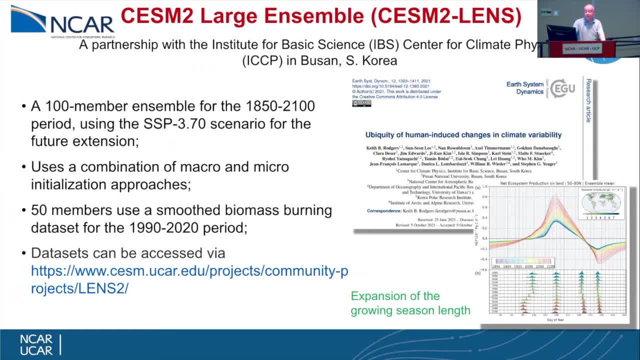 and this has been completed. this was a partnership with the institute for basic science center for climate physics in busan, south korea. they provided the computational resources. we have completed a 100 member ensemble for the 1850 to 2100 year period using the ssp 370 scenario. 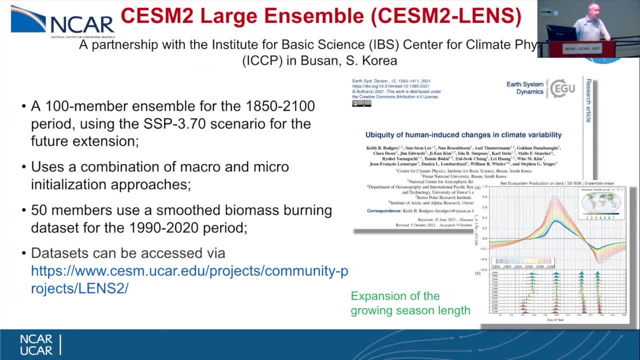 for the future extension. these use a combination of macro and micro initializations. micro is just simple atmospheric perturbation at restart and then macro is using different states for all component models, particularly the ocean component. we have 50 ensemble members with cmip emissions. you made six emissions for biomass burning. we also conducted another 50 members using a smooth 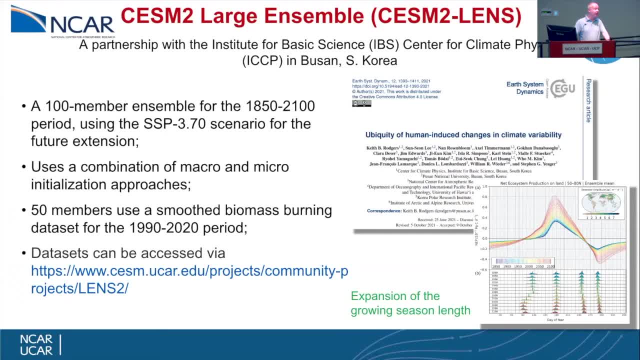 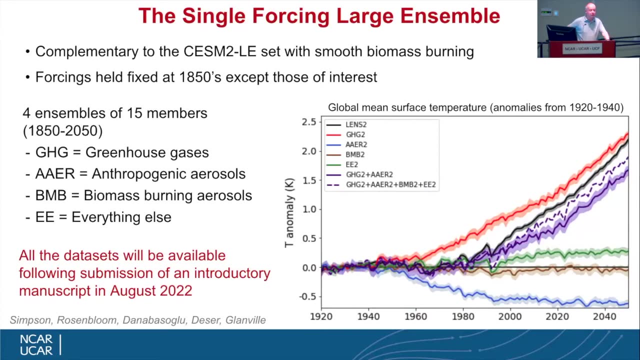 version of the biomass burning. all of these again are available at this website and, if you're interested in, the manuscript is given here. i suspect that this will be of use to quite many of you. a complementary set is the so-called single forcing large ensemble experiments. these use again the same setup as the csm-2 large ensemble but in these experiments 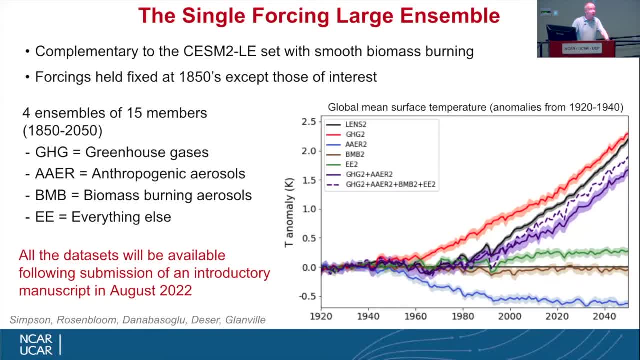 now we are fixing certain forcings and allowing only one forcing set to change. we have done four ensembles of 50 ensemble and we have done eight ensemble. we have done a hundred ensemble, 15 members each for the 1850 to 2050 period, And these are the greenhouse gas only. 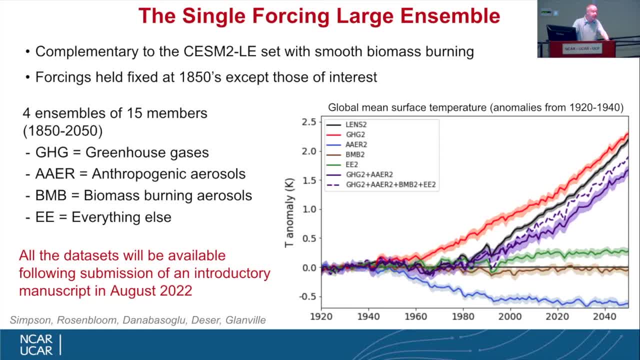 anthropogenic aerosols only, biomass burning aerosols only and everything else only experiments. So, for example, if you take the greenhouse gases, only experiment. in this case, the only forcing that's being changed is that forcing. All the other four things are staying. 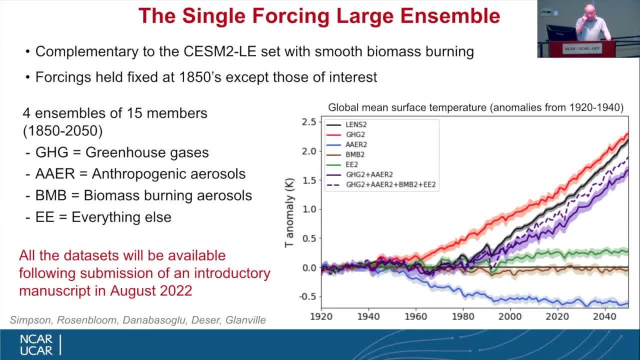 at 1850 levels, All the data sets. we are hoping that will be available by the end of this month. Isla Simpson is leading the manuscript. She's about to submit that And as soon as it's submitted we'll make all the data sets available. And the plot over here is showing the 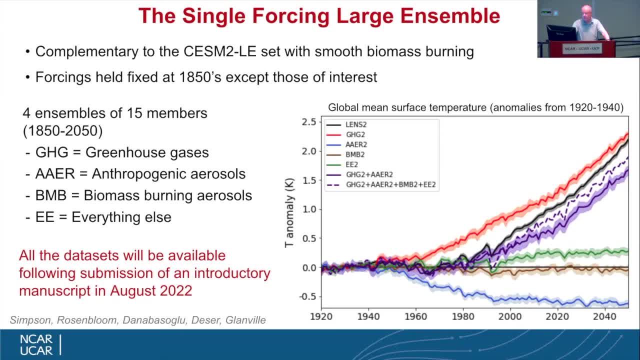 surface temperature anomaly time series with respect to 1920-1940 period. You can see the lens to large ensemble is the black line Here with the shading is showing, I think, one standard deviation or some measure of the ensemble spread And all the other individual forcings are given by different colors here And the dashed 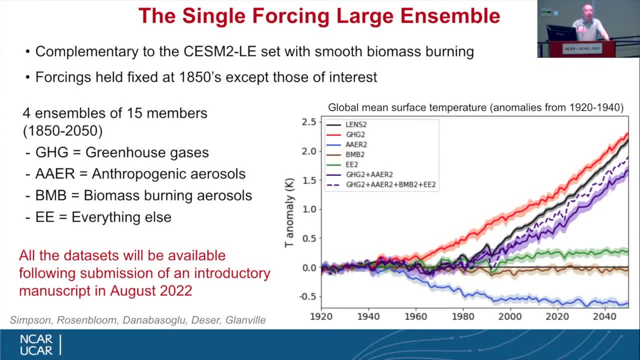 purple line is the sum of four only experiments. You can see that it's below the black line, So there is some non-linearity in the system. You are not recovering the full impact as shown in the lens to time series, And this is primarily related to non-linearities in the system. 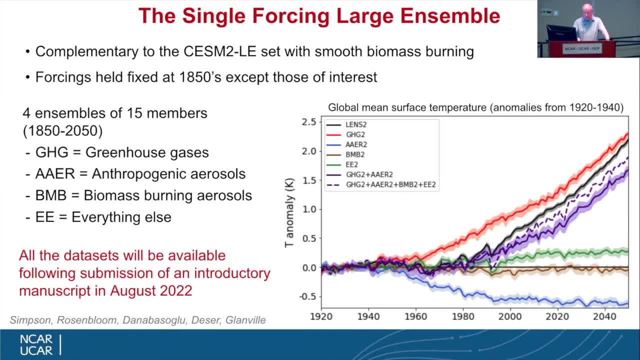 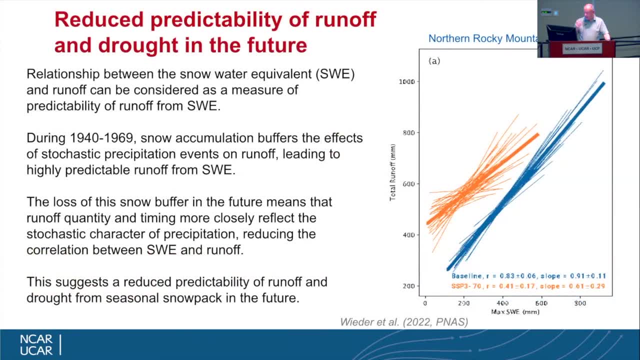 in particular, the mean state differences, And that's articulated in the manuscript that Isla is about to submit. Okay, This was an application of these large ensembles. This is from the land model working group. What is shown here is maximum snow watery coolant. 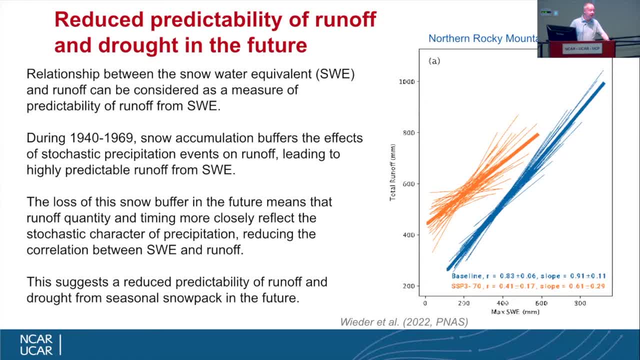 Plotted against the total runoff from these simulations. The blue lines are from the historical period And it is showing that during the 1940-1969, that's for that period- snow accumulation is essentially buffering the effects of stochastic precipitation events on runoff. 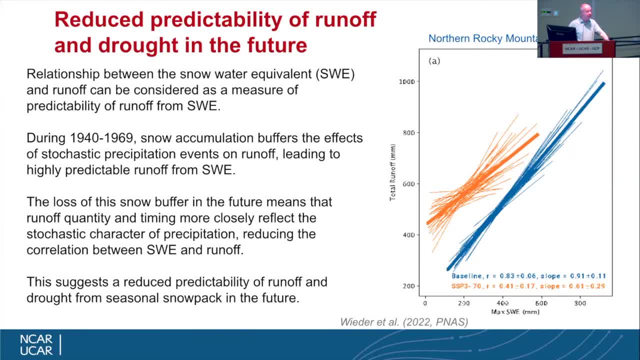 So in this case there's a clear linear relationship between snow, watery coolant and total runoff. But if you go to the future and those distributions or regressions are shown by the orange lines here, the situation changes. Because of the warming, the snow is melting and that buffer is lost. That means the relationship. 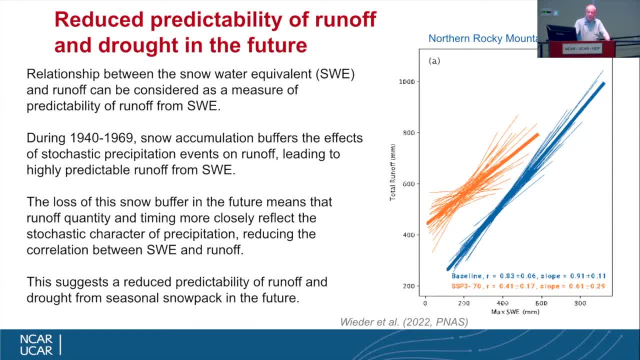 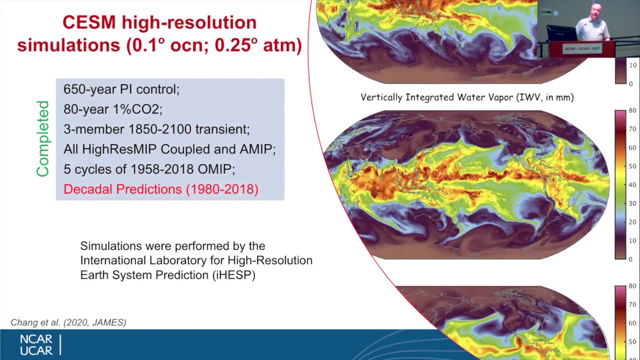 between precipitation and snow, watery coolant or the runoff, for example, is becoming less predictable. It is essentially reducing the predictability of runoff And drought in the future, primarily reflecting the stochastic nature of precipitation fields. About 10 minutes at most, right, Okay, So another effort that we had. I'm using head here. 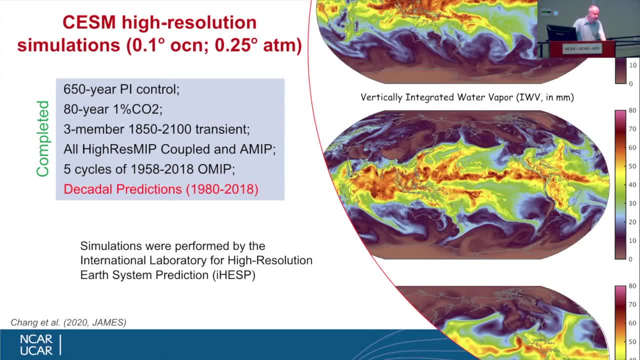 was the CSM high resolution simulations. These were using, or these are using, a tenth of a degree, nominal tenth of a degree ocean and sea ice resolution and quarter degree atmospheric resolution. And we have completed a 650-year PI control, 80-year 1% CO2 experiment, three members of 1850-2100. 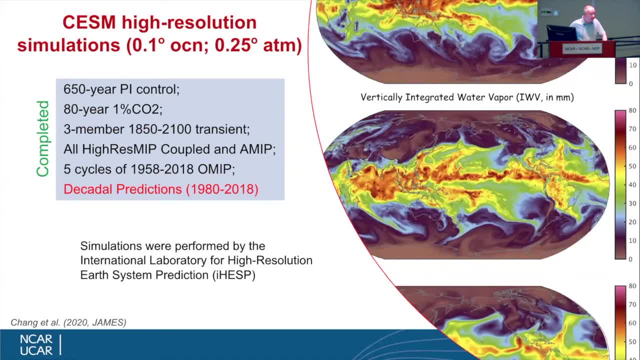 transient simulation. We have completed all of the high res MIB. that's one of the CMIP6 sort of satellite MIBs coupled and AMIP-type simulations. For those of you who are not familiar with AMIP, it's the Atmospheric Model Intercomparison Project and it is atmosphere-only simulations. 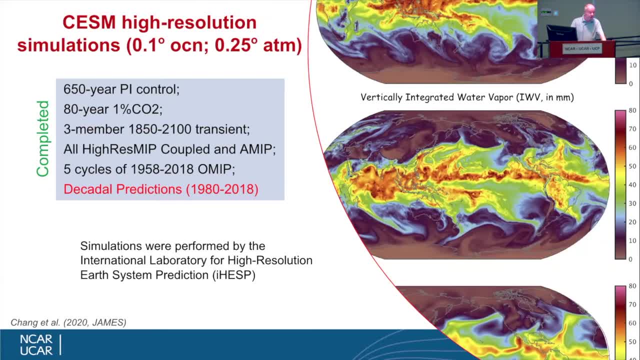 And we have also done five cycles of ocean-only experiments, that's OMIP for the 1958-2018 period, And we have also in the process- well, we have completed an initial set of decadal predictions with this high resolution system. It was a collaboration between Texas A&M. 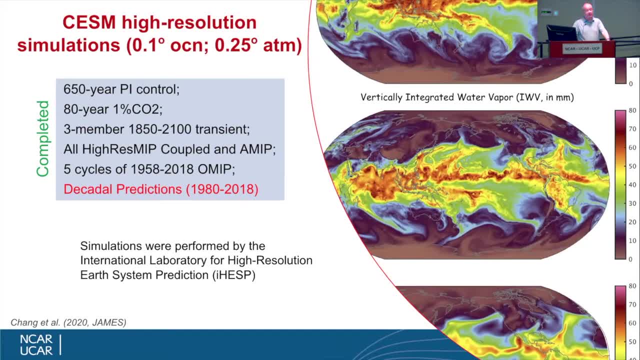 us and the Chindah National Lab for Marine Science and Technology, and it got terminated in December of last year. But all of these simulations are available. most of these are available to you if you are interested in looking into High Res simulations. 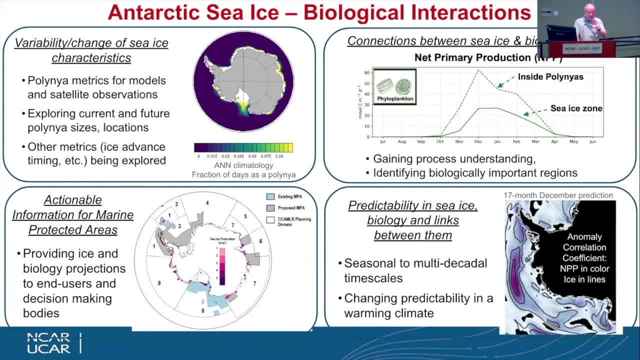 Okay, I just wanted to just mention that. coming back to the actionable science part that I mentioned, this is showing examples from our polar climate working group. They are looking into for, for example, in the Antarctic, interactions between Polinius and ocean biochemistry. 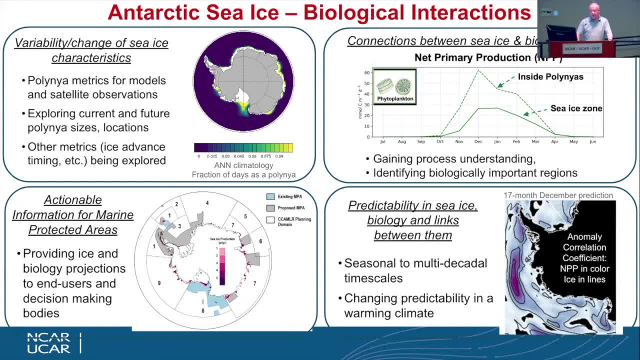 And just to show an example here, the lower left panel- they are providing sort of information for decision makers where the marine protect, where the future marine protected areas should be designated, as should be designated. We have some existing ones already and they are shown by the bluish colors here. 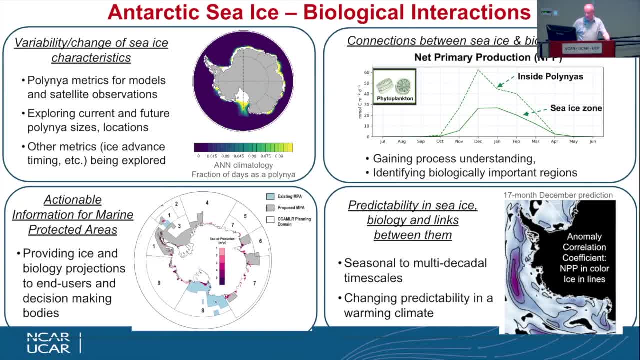 But the whitish regions, numbered from one to nine, are under consideration. So our polar climate working group, using CSM simulations, are trying to provide information as to which one of these regions should be designated Should be given priority in terms of being declared as marine protected areas. 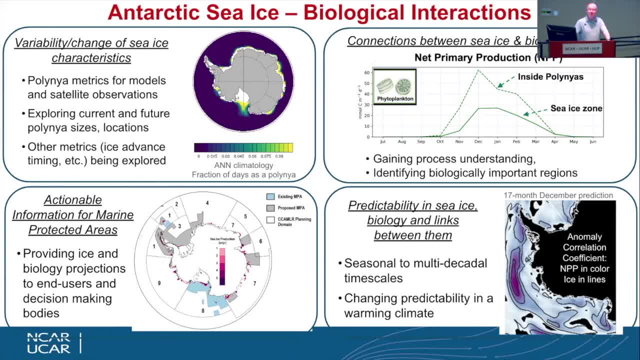 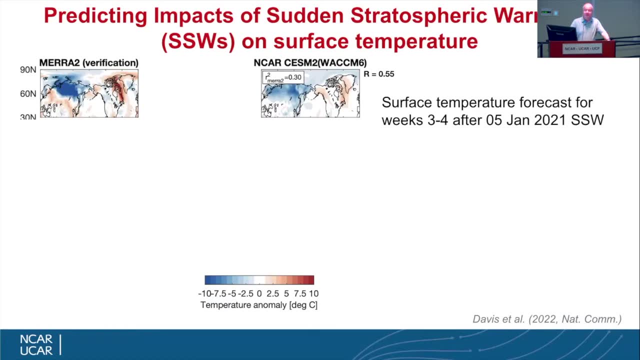 Of course, this requires agreement between, I think, 26 nations, and two of the nations are Russia and Ukraine, So this is going to be a major problem, I think, going forward. Okay, I mentioned predictions and I tried to distinguish it from projections. 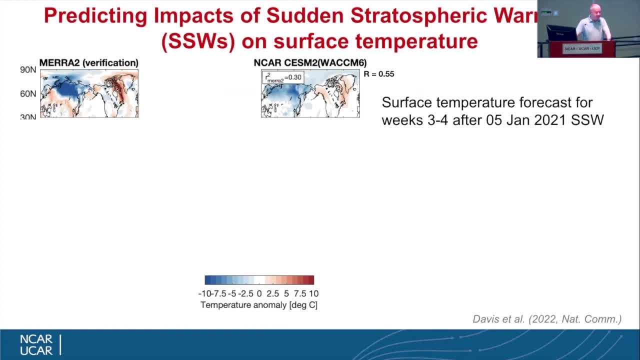 So we are using CSM for sub-seasonal- Yes, And for sub-seasonal prediction purposes, And this example is using CSM with the high top atmospheric component. That's the whole atmosphere. community climate model version six. What is shown here is surface temperature forecast for weeks three to four after January. 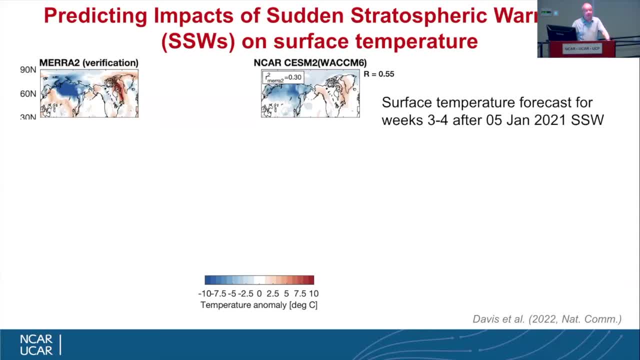 5th 2021, stratospheric southern warming event. I don't know, I don't expect you to be familiar with this event, but stratospheric southern warming events, Yes, It's associated with the breakdown of the polar vortex and they are thought to be impacting the surface temperature, particularly in the northern high latitudes. 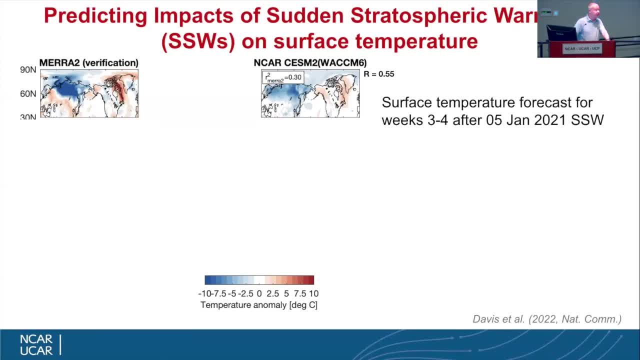 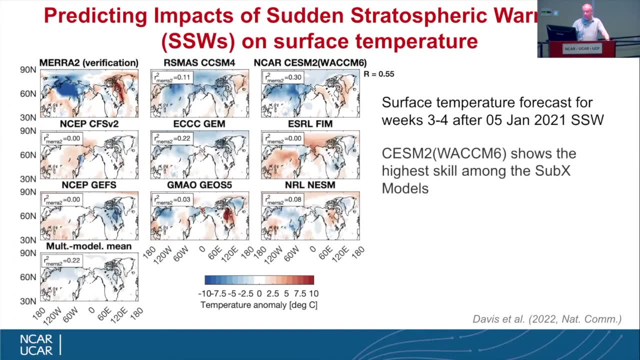 CSM simulation is shown in the middle and the verification is a reanalysis. product Meritude is shown on the left side. So we are doing quite well And in comparison with all the other models participating here. these are postage stem plots. 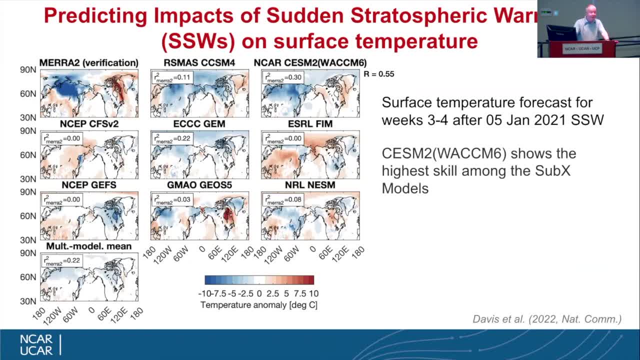 So I don't expect you to look at all of them in detail. You can take my word here: CSM is the best performing model in representing this warming feature in the northern high latitudes. But, more importantly, in this study led by Nick Davis, they showed that actually the common thinking is that the stratospheric sudden warmings are impacting the surface temperatures. 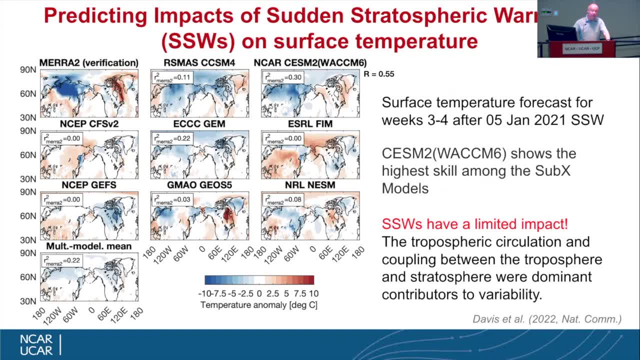 At high latitudes after three to four weeks. This study actually shows that that may not necessarily be the case. When they did- I mean the way they did it- they essentially changed their initial conditions. Some of them did not include stratospheric sudden warming events, yet they were able to produce the surface temperature signatures. 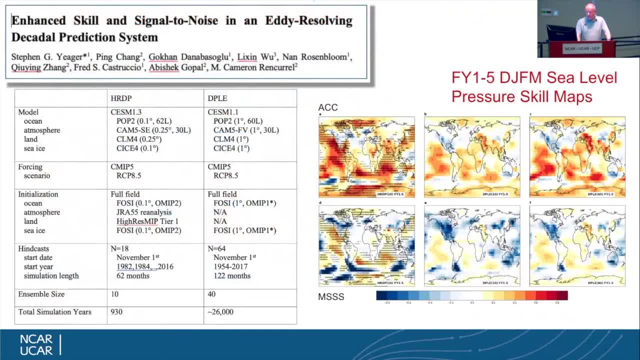 So I think that's an important finding. Another thing: I mentioned that we have the high resolution simulations. This is for decadal prediction, and what I'm showing here is one to five year average winter time. northern hemisphere winter time. sea level pressure skill maps. 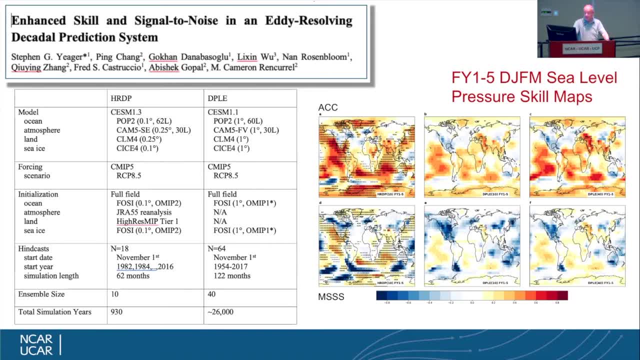 The top is for anomaly correlation coefficient ACC. the bottom line, bottom panels are mean squared skill scores, The point that I wanted to make here: the reds are good, the blues are bad, The left panels are from the high res. 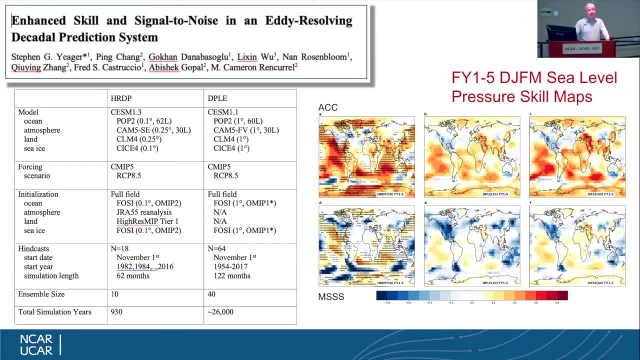 The middle panels are from the low res equivalent with similar ensemble member size- 10, and then the right side is low res with 40 ensemble members. The bottom line is that it looks like these are very preliminary. we are getting better skill with fewer ensemble members at higher resolution. 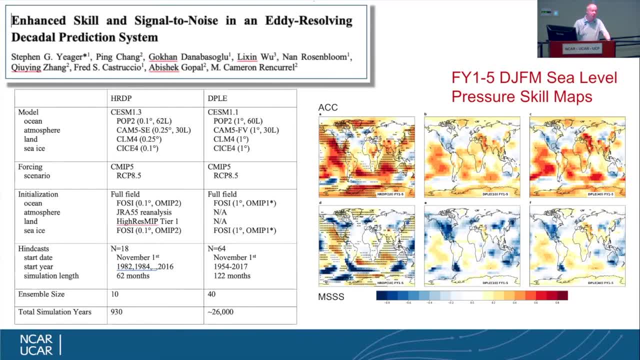 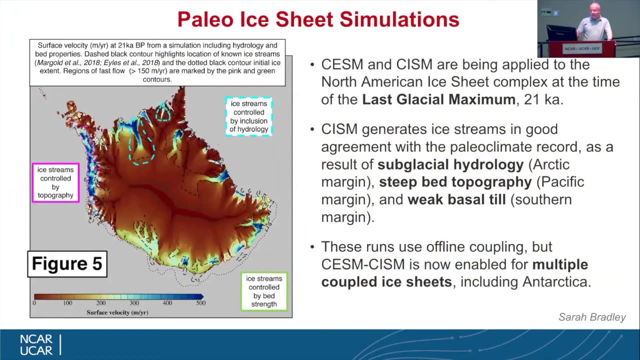 So it's improving the skill essentially, despite being more sort of- maybe chaotic is the wrong word here, But despite showing more variability, it's actually improved, being the atmosphere, ocean flux interactions, I will say I mean this was an example to show. 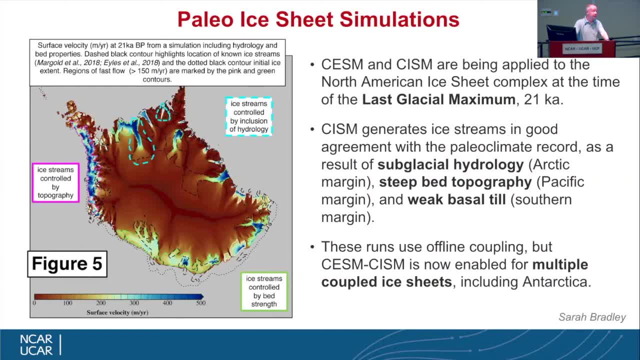 We have helio ice sheet simulations that are also ongoing, and this particular example is showing the Last Glacial Maximum North American ice sheet simulation, And we are now. even though this particular simulation is offline, it's still ongoing. CSM has the capability of now using interactive ice sheets and multiple ice sheets. We can do it. 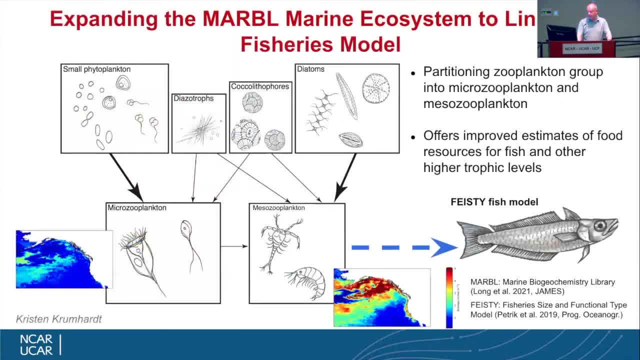 now with Antarctica as well as with Greenland, And we have just recently expanded our ocean biogeochemistry model. We use the MARBL framework for this purpose. We have now included a second zooplankton type and that is particularly useful for fisheries models. We are using the 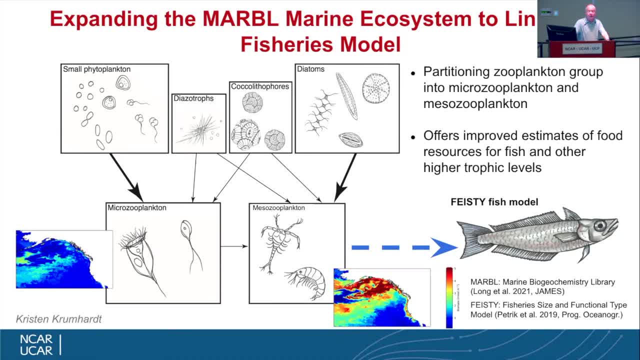 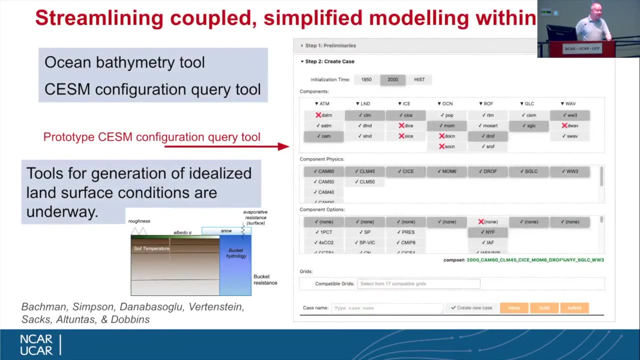 FeisteFISH model offline at this point, but we are in the process of bringing that particular fish model online. That will be a CSM component, but this is still ongoing work, if you're interested. Talking about simplified models, I talked about increasing model complexity. 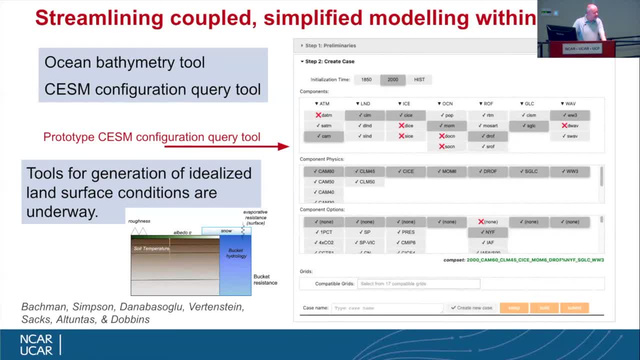 We can talk about this in future. which beорaking examples talk about the use of liquid permanency. We have a project- it has been going on for the last three, two and a half years or so. we are trying to provide easy to use, simple model or simpler model configurations of CESM. 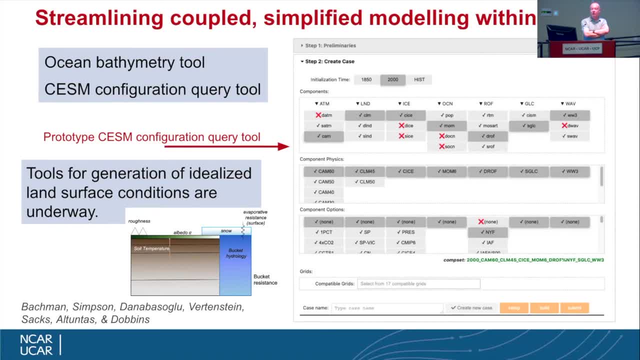 And I believe Ayla will be talking about this in more detail- I don't know which day, but one of these days- And we have actually created a graphical user interface for the user to easily set up a particular CESM configuration with just simple push of buttons. 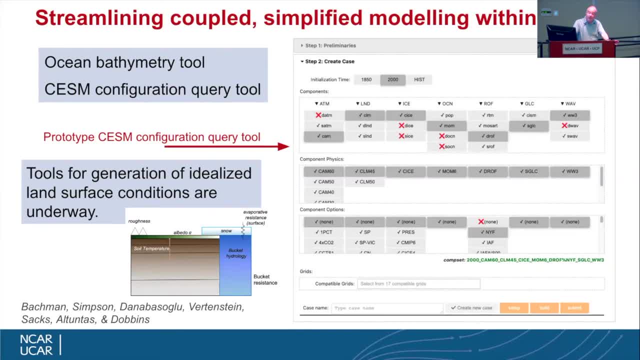 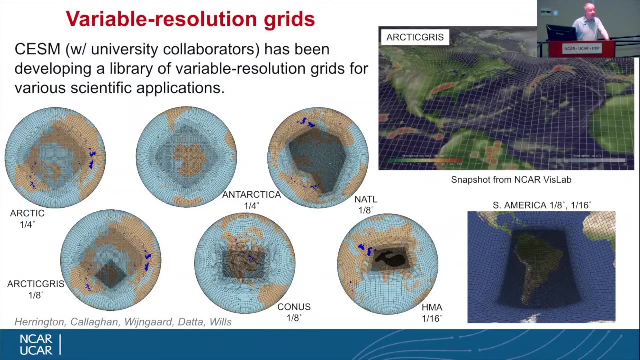 So we think that this is going to be quite useful. We are at the trial stage with our some Unipig users, collaborators, but I'm hoping that this will be available to the broader CESM community. Okay, we have versions. We have the Microsoft variable atmospheric model. 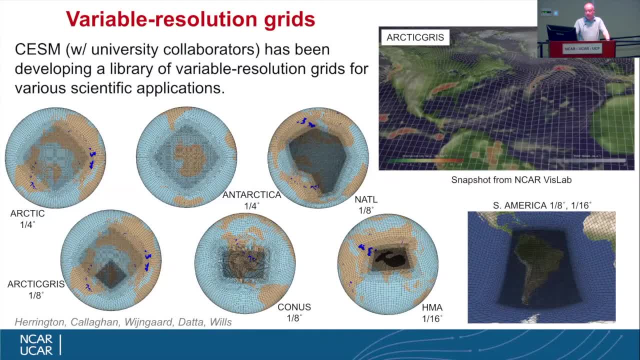 This is with the spectral element dynamical core. These simulations or these configurations are created by our university collaborators. You can see our existing grids. We have a high resolution Arctic grid. One of the most popular grid is the Conus grid. It's the one in the bottom row. it's the middle panel. 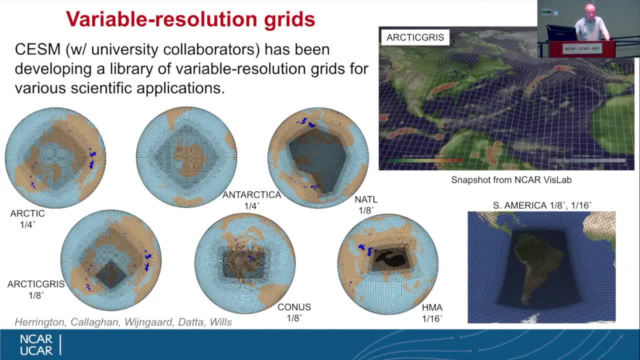 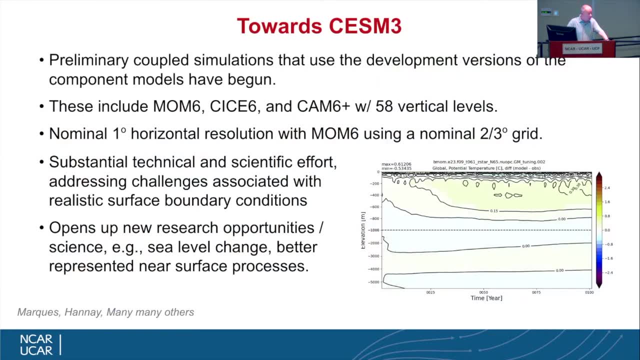 It's essentially increasing the resolution to one eighth of a degree over the continental United States. Just final slide. We are working on creating a new version of the model. I labeled this slide as towards CESM3.. We have preliminary coupled simulations that use developmental versions of the component models. These, as many of you may know, the older version of the model. 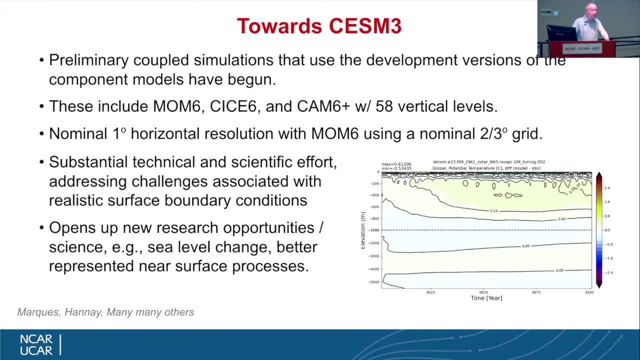 used the parallel ocean model. This is the parallel ocean program, version 2 for the ocean, That's POP2.. We have switched to MOM6.. That's a GFDL model, a modular ocean model, version 6.. So that's the new model. 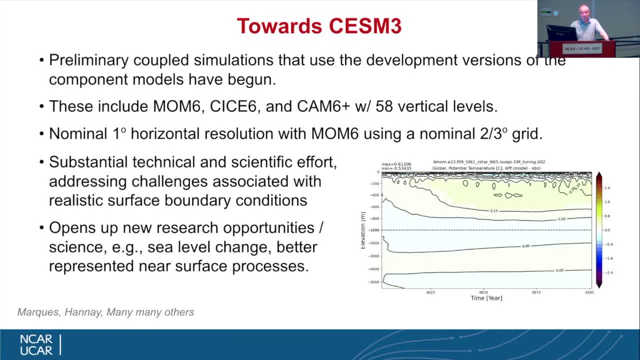 CI6, it uses CI6 and it uses the development versions of CAM6 with. we are also increasing the number of vertical levels in the atmosphere. This is with 58 vertical levels, but we are hoping that the workhorse model will use about 92.5.. 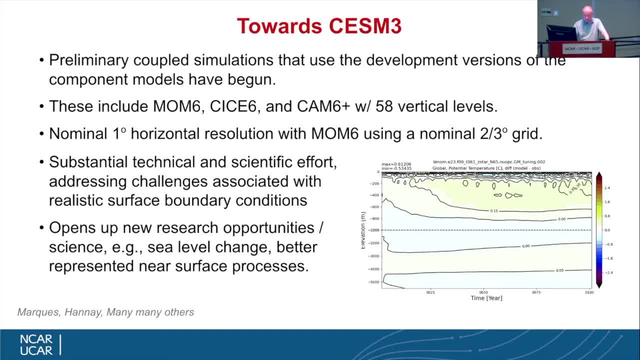 And we will use about 92 vertical levels in the atmospheric component. Needless to say, each time we develop a new model it is both a big scientific and technical challenge. So it has been taking us quite a while and it will be probably- we hope- to get some preliminary results by summer of next year. 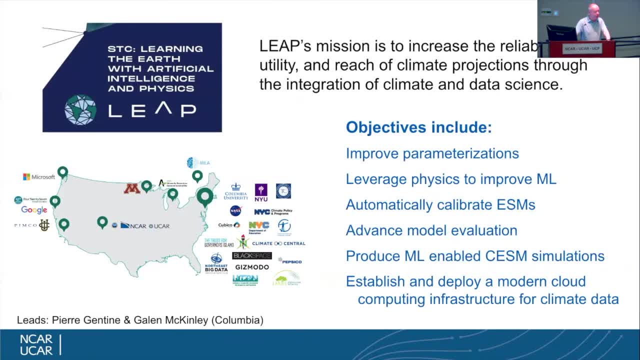 With respect to sort of future work, we are collaborating with the LEAP Science and Technology Center, that is, the learning the earth with artificial intelligence and physics. This is going to bring many machine learning, artificial intelligence aspects into the CESM. So CESM is going to be the primary coupled system in this effort. This is led by University of Columbia. 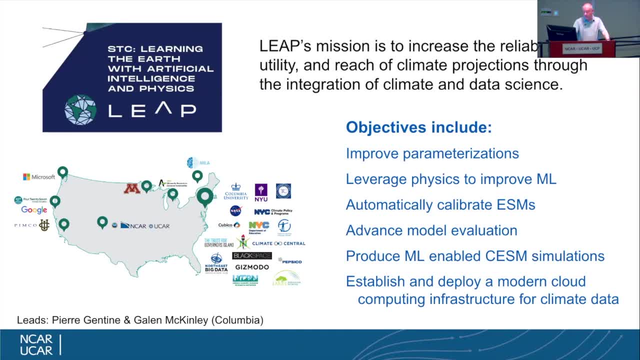 And it has many partners: the university partners and private partners as well. So this is going. I'm looking forward to this particular project effort to bring in machine learning aspects. We also have a few other projects, such as M2Lines. that's focusing on bringing machine learning into the ocean, the new ocean component, MOM6.. 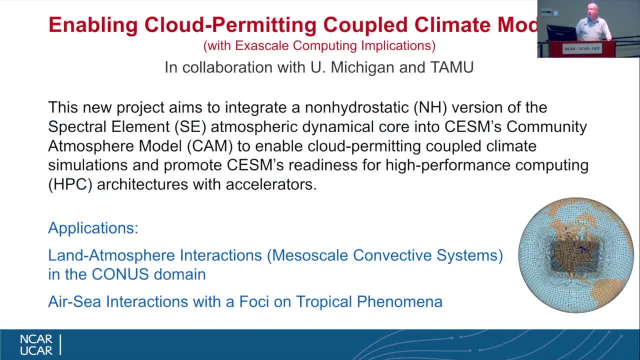 And finally, we are about to get started on this project, which will be still five months, I think We are trying to do enabled cloud permitting coupled climate modeling. The target resolution would be three kilometers or so within the coupled system And the idea is to incorporate a non-hydrostatic dynamical core with the spectral element dynamical core of CAM. 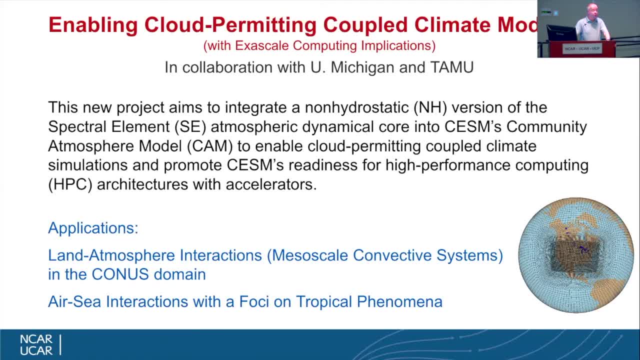 This would enable us both. This would bring in both Fortran and C++ Versions of the model And in that case we can take advantage of the GPU side of the DRECHO, the new computer system that's supposed to be on the well. that's supposed to be coming, hopefully next year. 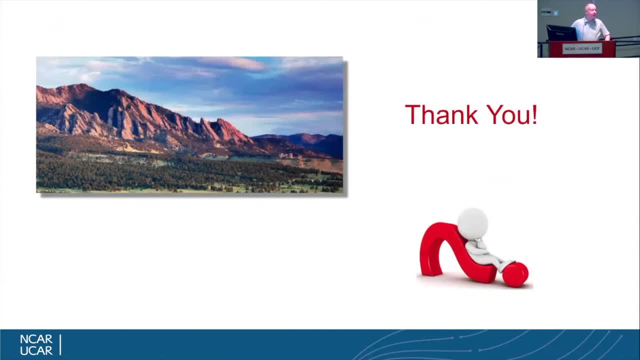 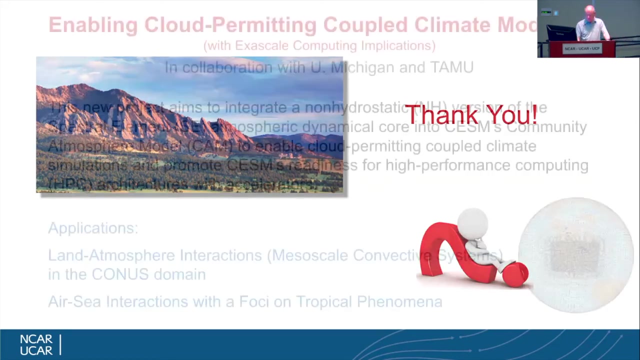 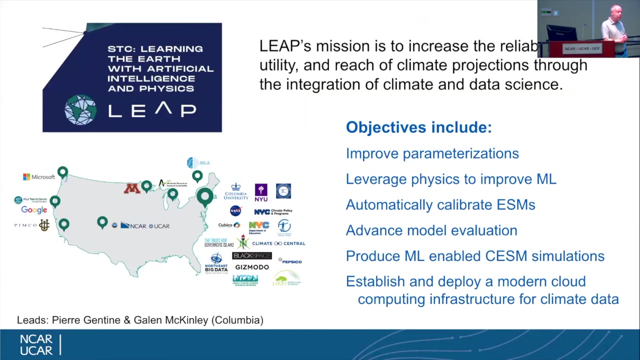 So with that, I'll stop up and hopefully take questions. I know that I'm almost too much time, Thank you, Do you have any questions? Well, thank you, Yes, Well, so yeah, I mean that's a good question, because many I mean. 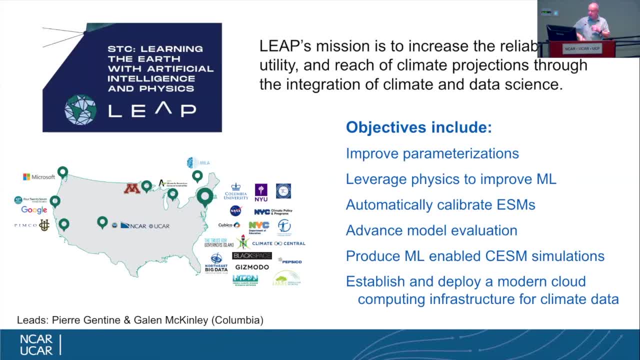 there's some. there are some challenges, of course. So I didn't go over the objectives. Maybe I should just briefly mention that the objectives of this proposal- The first one is, I think, important- improve parametrizations. So they will be looking at both atmosphere and land also, and ocean. 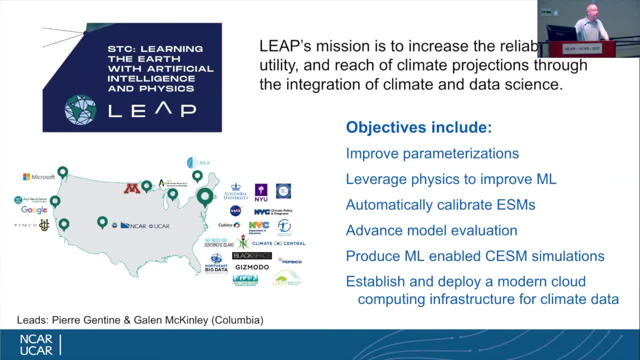 They will try to look at. if there are aspects of elements to improve existing parametrizations And By machine learning techniques, one idea could be to replace the existing parametrizations with their machine learning equivalence. This can be, I mean, through emulators and all that stuff. 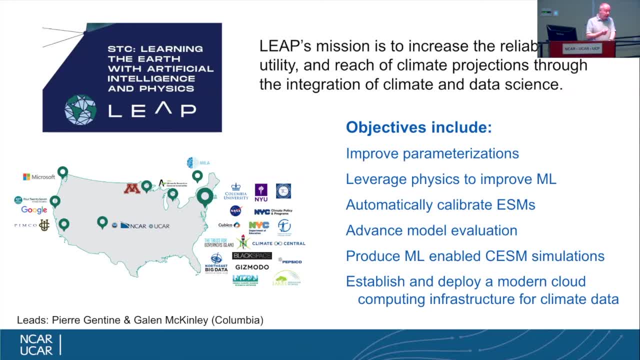 So they are. they are. if that can be achieved, then they're supposed to be cheaper, first of all to run. Then the second aspect is that those Machine learning based parametrizations are better suited to run on GPU based systems. 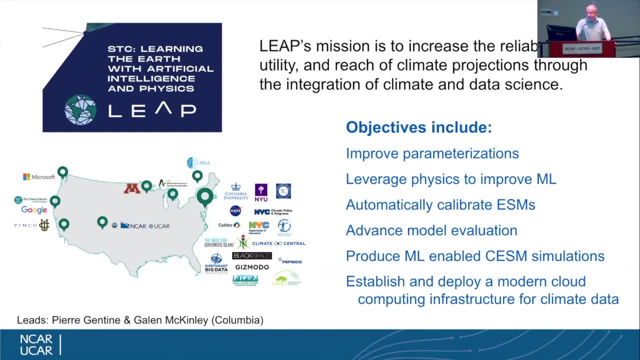 So that would be sort of the two advantages. But of course you can't just trust these as black box models. So that's why I mean the NCAR collaboration with this particular group is quite important, because we will be jointly evaluating making sure that they are physics based and they are doing what they are supposed to do. 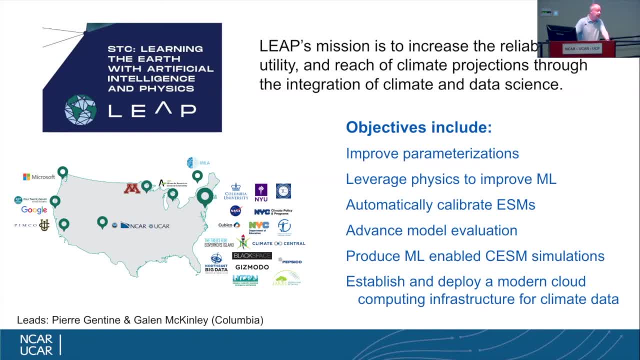 And then we are going To also provide our expertise from the climate modeling side, and it's not an easy adventure. I mean then also, it can be used, for example, leverage physics to improve machine learning techniques as well. So it is, it is a complicated effort. 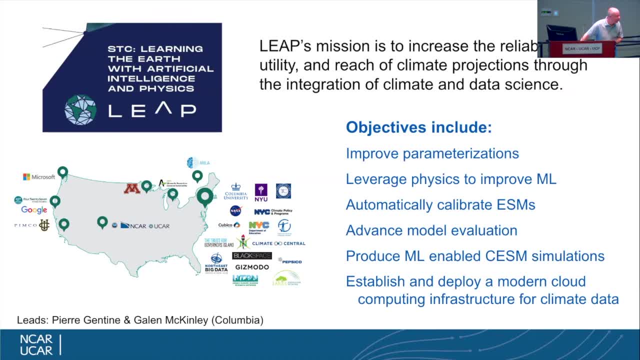 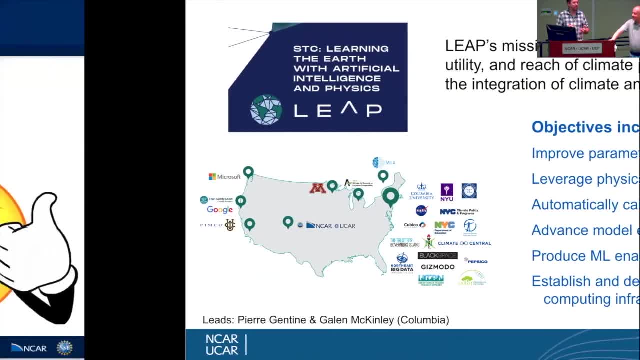 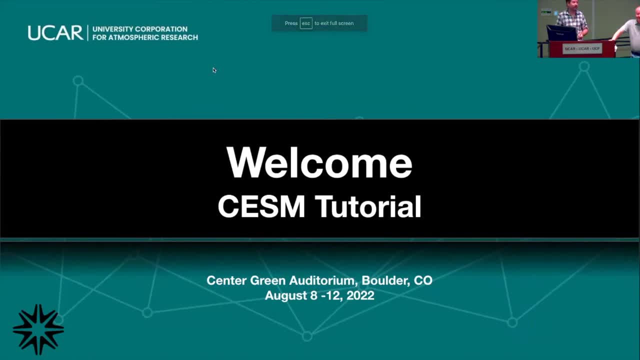 I do land use, land cover change and I'll be presenting some later, But one of the things to understand is this is a community model, So you're not expected to have understanding of absolutely every component of this model. As we go through this tutorial, you will learn about things that are outside of your domain. 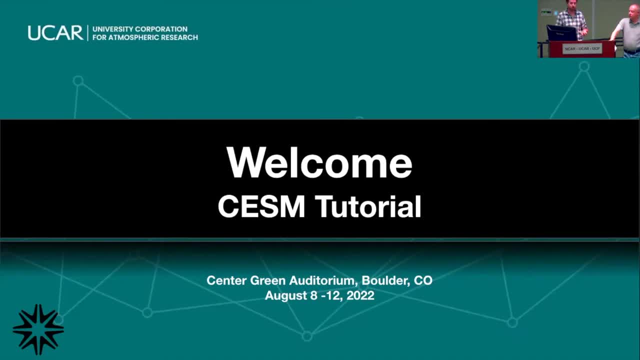 of expertise and your understanding, And that's fine, because what you will be able to see is this tool that can answer really complex questions about the future and the past and our current climate and how to use them for your research. As Gokhan showed, it's not just a matter of running the model. 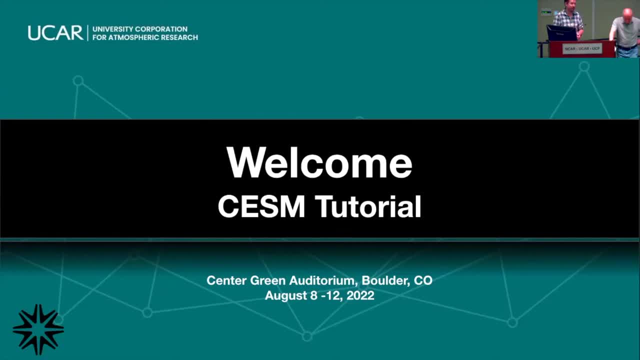 We have a large amount of data that's already coming out of the models we've run. So your research may be running the model, setting up experiments. It may be processing other models that have already been run. So, as you go through this week, don't feel like it's a competition. 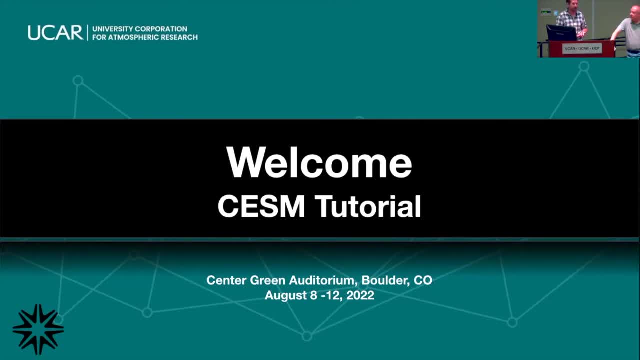 You don't have to be competing against everyone to show how much knowledge you have. What it's really about is learning, and it's learning how these tools can be useful in your research context, And with that, I think we'll go to the break.